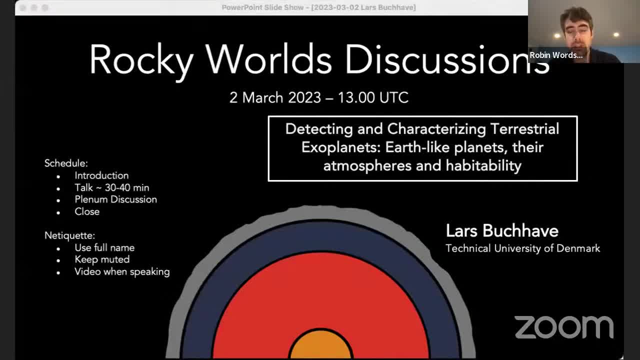 Okay, so today's speaker is: we're happy to welcome Lars Lars Bukhava. Lars is a professor at the National Space Institute of the Technical University of Denmark and he works on the discovery and characterization of exoplanets, including their composition and internal structure and atmospheric properties. 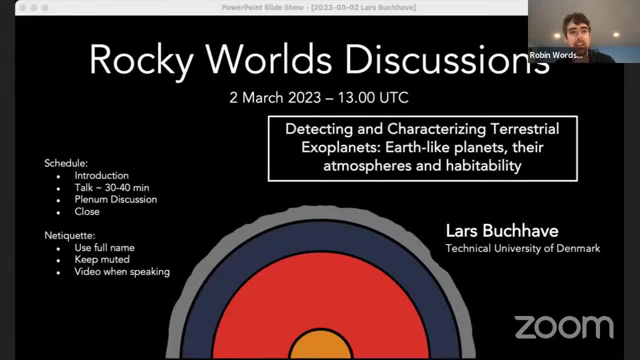 Some of his notable work in the past has revealed the links between planet occurrence and host star metallicity, but he does a whole bunch of other things besides that as well, And so today he's going to be talking to us about the detection Of exoplanets. 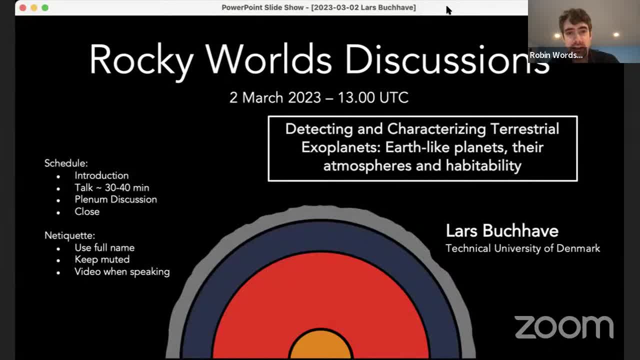 Detection and characterization of terrestrial exoplanets, with, it sounds like, a particular focus on Earth-like planets, including their atmospheres and habitability. So over to you, Lars. Thank you so much. Should I try to share my screen? I will stop share. 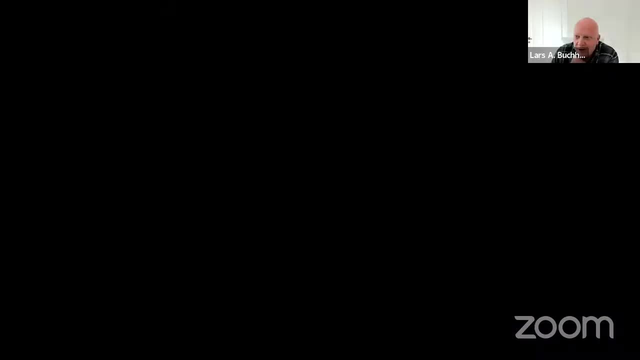 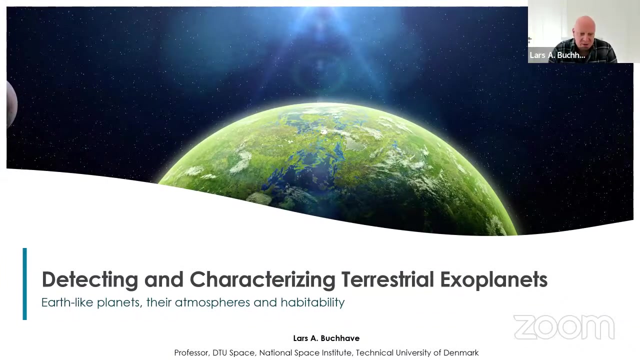 All right, Go ahead when you're ready. You see this this over here Looks good, All right. So yeah, thank you so much for the invitation to talk today. as you said, I'm Lars Bukhava. I'm a professor at DTU Space. this is the National Space Institute at the Technical University of Denmark. 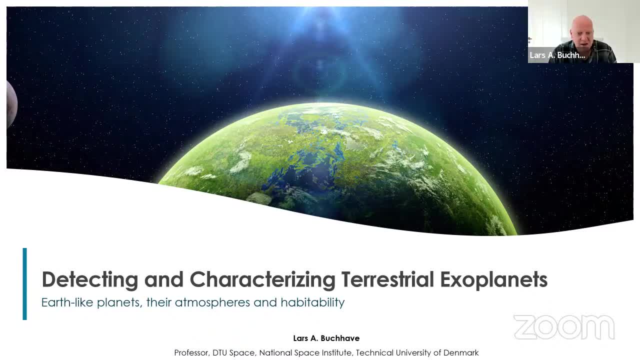 And yeah, the title of my talk is Detecting and Characterizing Terrestrial Exoplanets. So I mean the last 30 years of exoplanet, almost 30 years of exoplanet research, has revealed a ton of different exciting discoveries, of course, 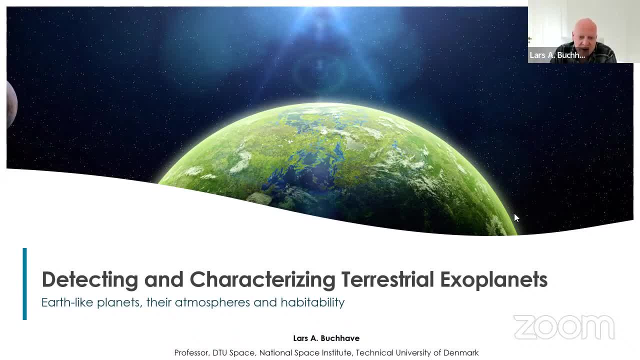 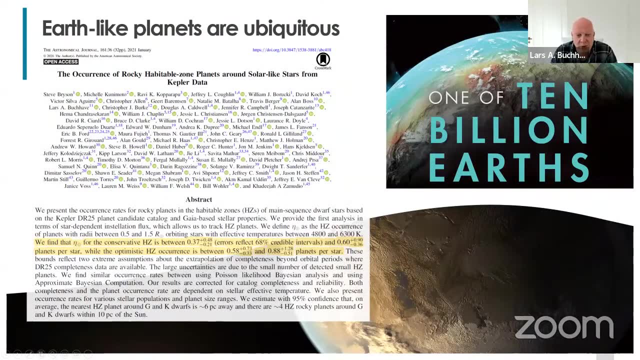 But if I were like pressed to come up with one single thing I think is exciting, it would probably be the fact that small planets have turned out to be incredibly common, And so there's, of course, a number of different, many, many different papers on this. 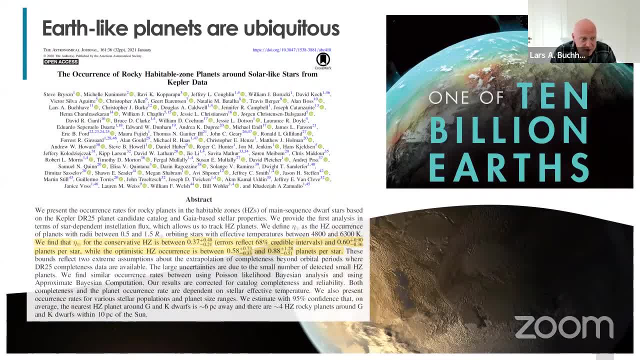 I've highlighted one here from a few years ago by Steve Bryson, led by Steve Bryson. So basically this is a Kepler mission legacy paper, I would call it, where Steve and team looked at the occurrence rate of the exoplanets. So basically this is a Kepler mission legacy paper- I would call it- where Steve and team looked at the occurrence rate of the exoplanets. So basically this is a Kepler mission legacy paper- I would call it- where Steve and team looked at the occurrence rate of the exoplanets. 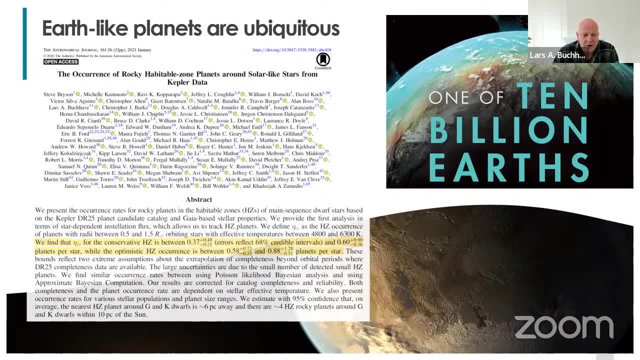 habitable zone, earth-sized planets orbiting solar-type stars, By also doing an injection and recovery test in the Kepler data, And so this elusive E to Earth is being assessed here, And there's a few numbers here, highlighted in yellow, and I'll try to unpack them just a little bit. 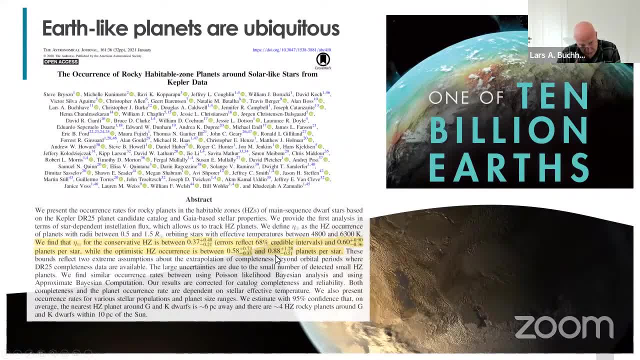 It's not been too long on this, but basically it depends on the four numbers, depend on how you extrapolate the data, if you're conservative or you're conservative, And there's a few numbers here highlighted in yellow, and I'll try to unpack them with just a little bit, not spend too long on this. but basically it depends on the four numbers, depend on how you extrapolate the data, if you're conservative or you're conservative or you're non-conservative. 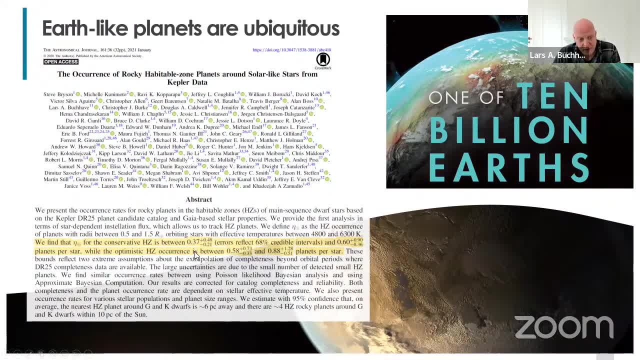 very optimistic And there's also two different habitable zones: the conservative habitable zone or the optimistic habitable zone. So if you take the most conservative extrapolation and the conservative habitable zone, this paper comes this conclusion: is that about 0.4, there's about. 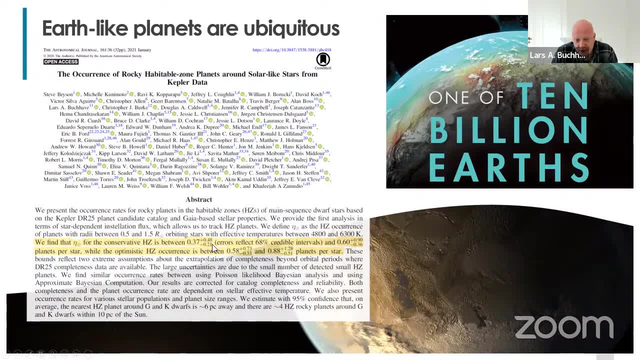 0.4 Earth-sized planets in the habitable zone orbiting solar-type stars, with some fairly large uncertainties, of course. If you go to the other extreme, the most optimistic extreme, the number comes to 0.9, with also sort of large uncertainties. But the point here is that this number 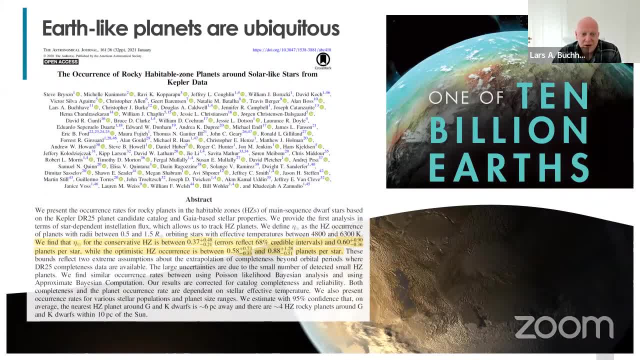 is very large. I don't think the final word has been said on the exact occurrence rate of each Earth or habitable zone, Earth-like planets around solar-type stars, But the excitement here to me is that that means that there's really many, many of these planets in our astronomical backyard. 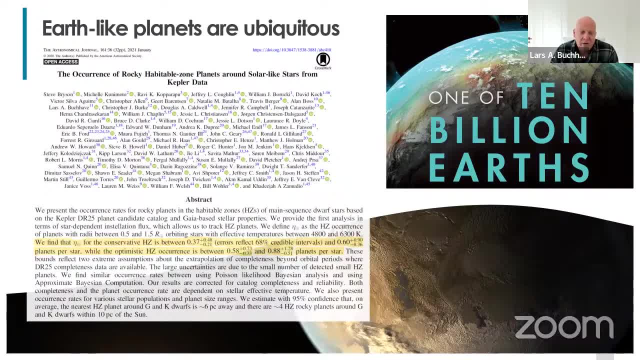 meaning that we can analyze, detect and characterize these planets because we have the required amount of photons. Conversely, if this number was tiny, we would have to look very far away to find these planets. But this is, to me, what excites me about the 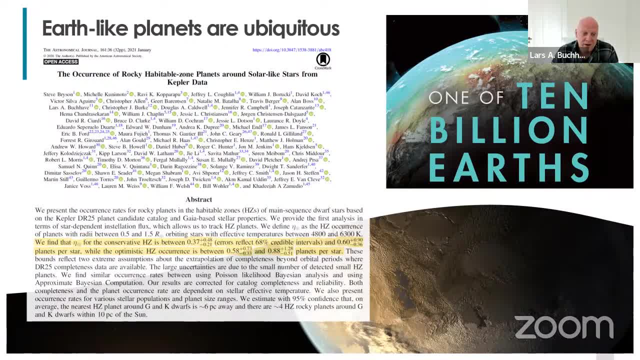 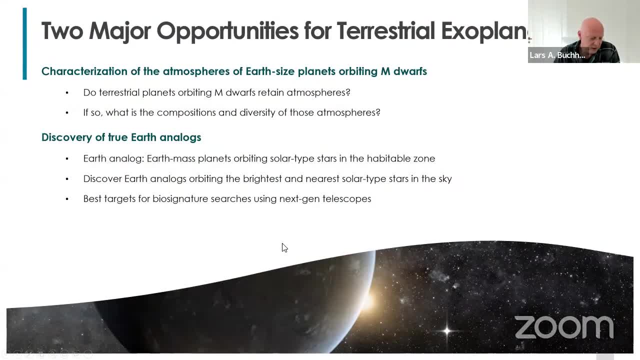 coming decades is that this number is fairly large, so that we can really dig into the planets in our astronomical backyard. So our group, I think, is focused. we're really excited about the small planets. This is very difficult work, but we're kind of focusing on two, what we see as two. 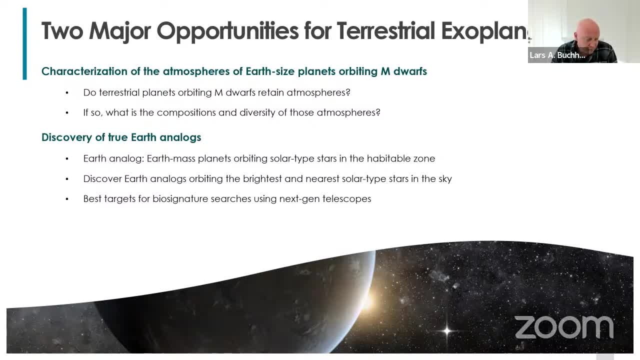 Earth-sized planets. So one is the possibility of characterizing the atmospheres of Earth-sized planets, of course orbiting cooler M-dwarf stars, with James Webb and other instruments that are coming up, which I find is extremely exciting. This is the first time we potentially have access. 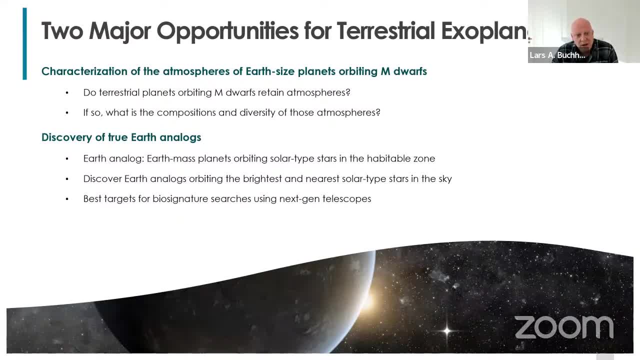 to do this, to really characterize secondary atmospheres around terrestrial planets And the other. the other area we're interested in is really trying to discover a true Earth analog, so basically Earth-sized planets orbiting solar-type stars in the habitable zone, And this is, of course, 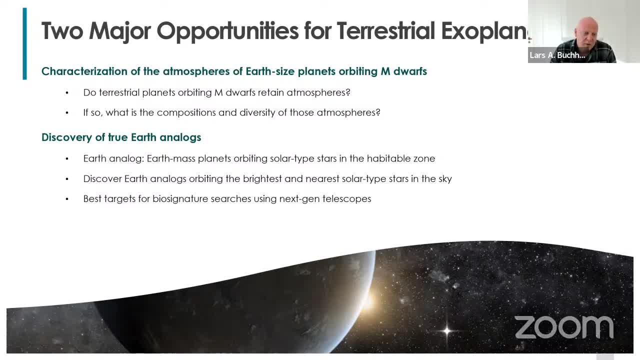 extremely difficult and elusive, but one of these things that will lead to these next generation telescopes that want to look at the atmospheres of true Earth analogs and search for biosignatures in their atmospheres. So, if we talk about the first area, 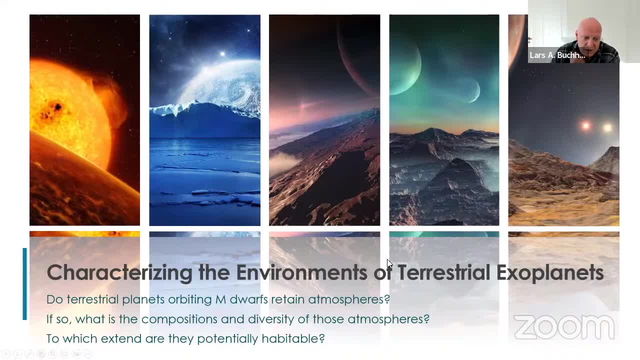 characterizing the environments of terrestrial planets. the opportunity here is that we can now, for the first time perhaps, look at a secondary, highly molecular weight atmosphere orbiting an M-dwarf, a planet orbiting an M-dwarf, And of course this is a very different environment than 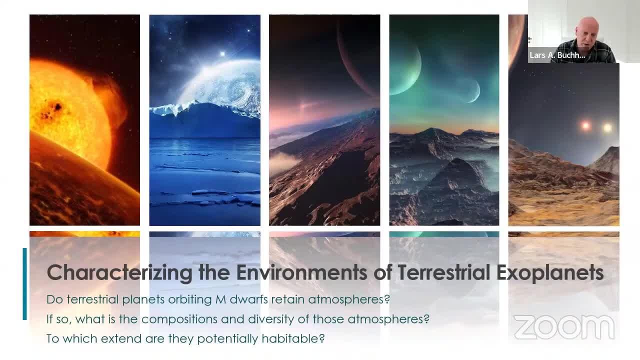 the solar-type stars. The planetary systems are very compact, usually packed systems, and the proximity of the planets is much closer to the host star than in the solar system. And we also know that M-dwarfs have a very young active phase. They have a very young active phase. They have a 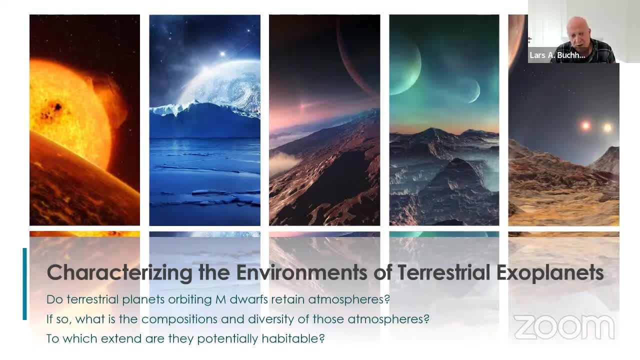 lot of flaring and so on and so forth in UV in the early stages. So it's likely that some of the close-in planets will have their atmospheres eroded over time. But it could also be that some of the planets further out perhaps retain their atmosphere and are maybe able to replenish them over time. 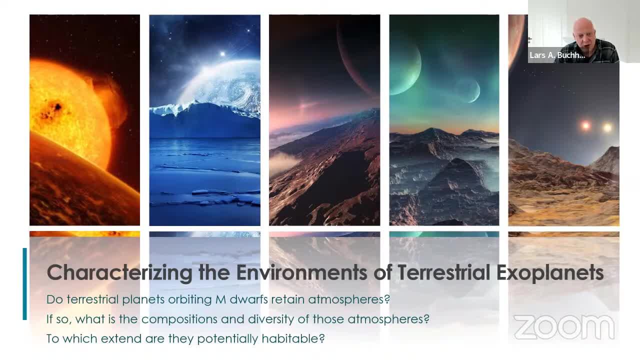 by outgassing or other volcanic activity or outgassing from the interior. So the zero thought question is basically, I would think, is: do any of these planets retain atmospheres at all or replenish their atmospheres around M-dwarfs, And where is? 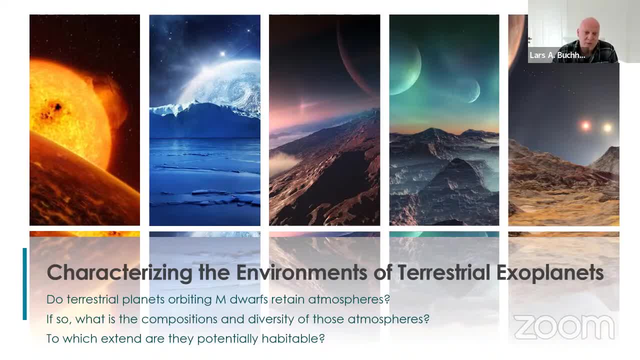 that kind of transition from planets that have lost their atmospheres to planets that actually have atmospheres, And if there are some of those planets that do retain atmospheres. the next question, of course, is what is the composition and diversity of these atmospheres? I find that truly exciting. I mean, we know that terrestrial planets in our solar 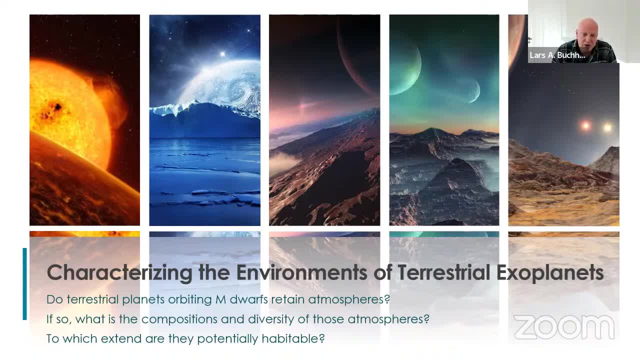 system, and just among those we have a very wide range of environments, from Venus, with this 100-bar CO2-dominated atmosphere and 500 degrees centigrade on the surface, to the Earth and then to Mars, with a very thin CO2-dominated atmosphere. 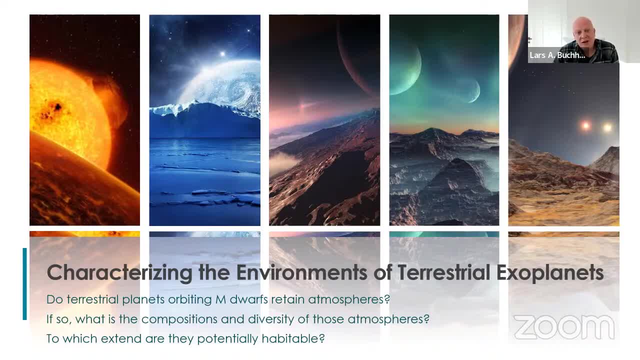 And of course, the next then question is: to what extent are atmospheres of terrestrial planets habitable, or are they at all? So for me, this is really very exciting- having been in this field some time now- that we're actually potentially able to study these secondary atmospheres. 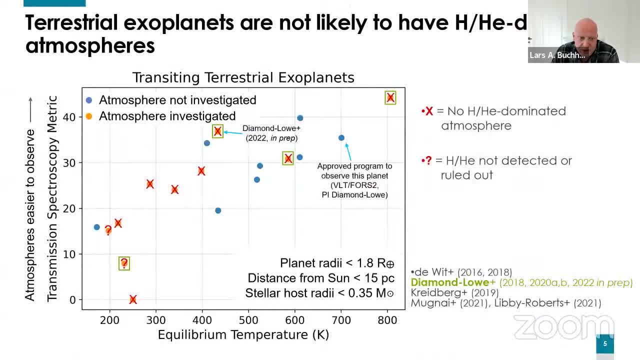 For the first time, of course, there's been work that's gone into this before James Webb was launched, with ground-based observatories and the Hubble Space Telescope in particular, And I'm showing here sort of a plot of the equilibrium temperature of small planets below 1.8 Earth radii. 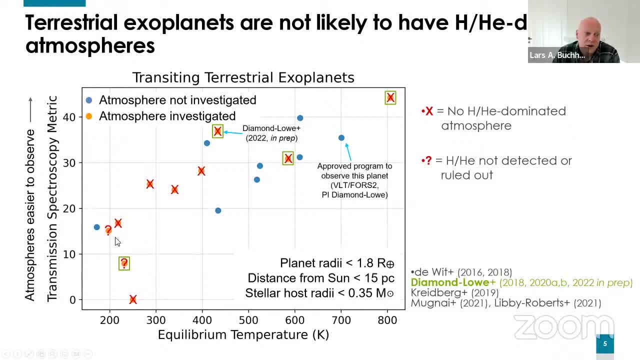 that are close to us and the transmission spectroscopy metrics on the vertical axis. So, basically, planets up here are easier to observe and our postdoc in our group, Hannah Diamond Lowe, has been one of the people pioneering this work and trying to rule out the existence, or rule in the existence of a hydrogen-helium-dominated 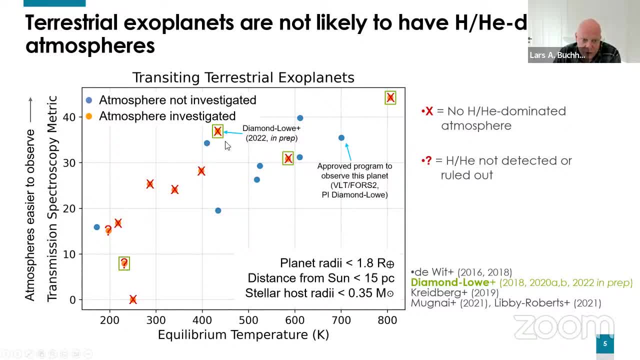 atmosphere around these small planets, And so you can see in this diagram, the ones with red frosses have been determined to not have sort of these hydrogen-helium-dominated atmospheres. Maybe that's not super surprising that planets are unable to hold on to a hydrogen-dominated atmosphere, But in any case, 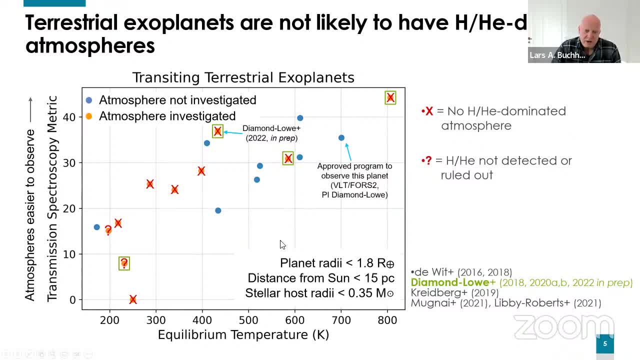 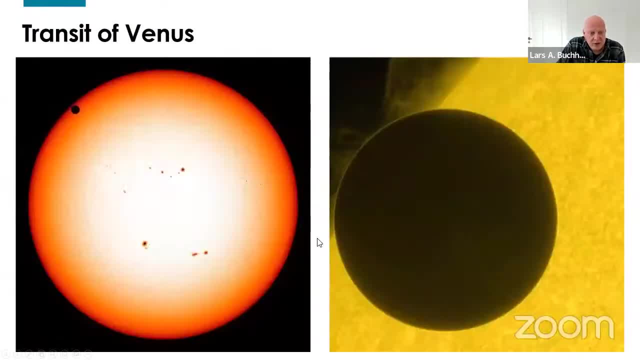 most of these planets that have been expected don't have these extended atmospheres. Just to sort of put it into perspective, I kind of like this slide, which is basically Venus eclipsing the Sun up here on the left, and then that close-in actual picture of Venus And, as you 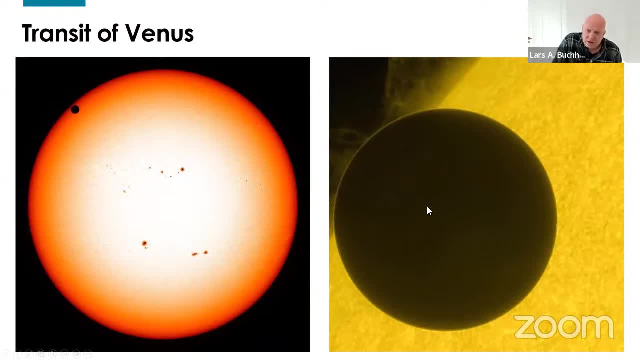 know, Venus is about the size of the Earth, So we're about, you know, 6,400 kilometers in radius And the atmosphere of Earth is, you know, 99% of the mass is within 100 kilometers. And so what? 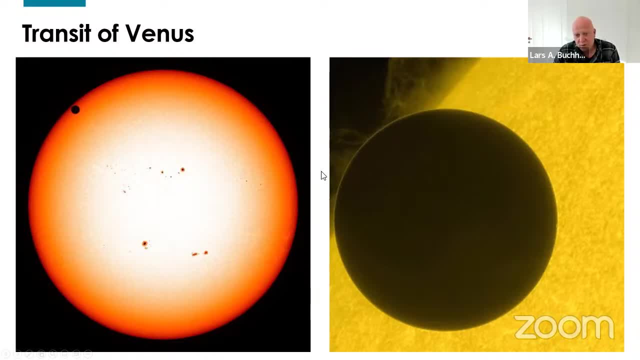 you're seeing here is this very, very thin outline on Venus, an assumed-in picture of the atmosphere of Venus, And what we're really trying to measure here is the size of that atmosphere as a function of wavelengths to get the transmission spectrum, And that is excruciatingly difficult, But it just 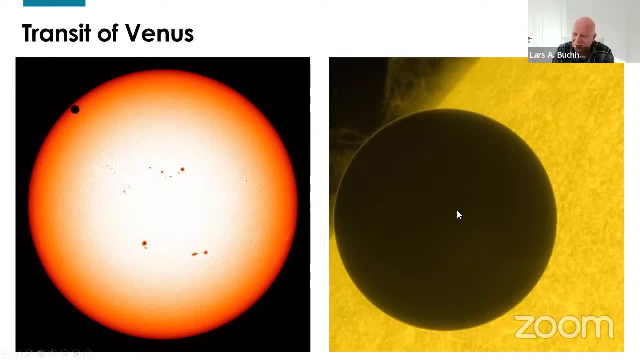 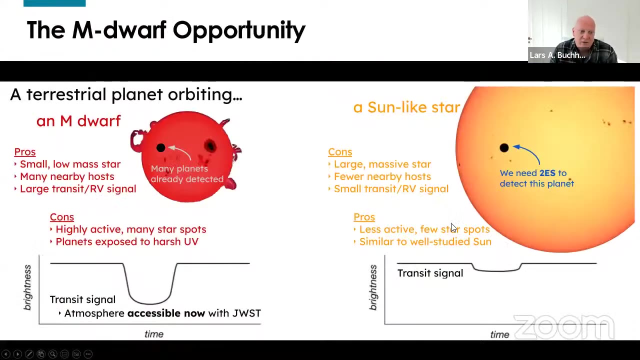 sort of seeing this picture reminds me basically of the difficulty of this task. And then you know, you of course have stellar activity and spots and so on and so forth, interfering with the measurements. This is really truly very, very difficult, But we do have the opportunity of 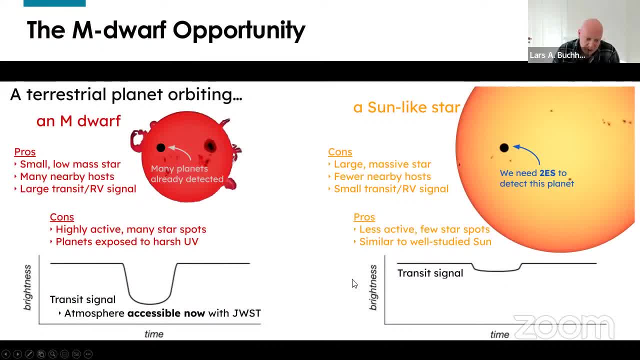 observing these terrestrial planets around M dwarfs And of course, as you know, that means that we just get a much larger transit signal compared to if the planet was orbiting or transiting a solar-type star. These types of stars are really not within reach, I think with James. 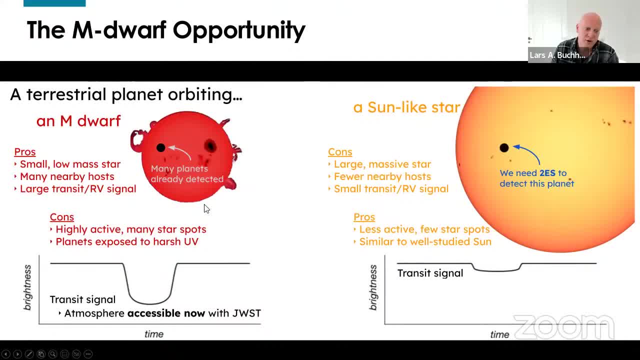 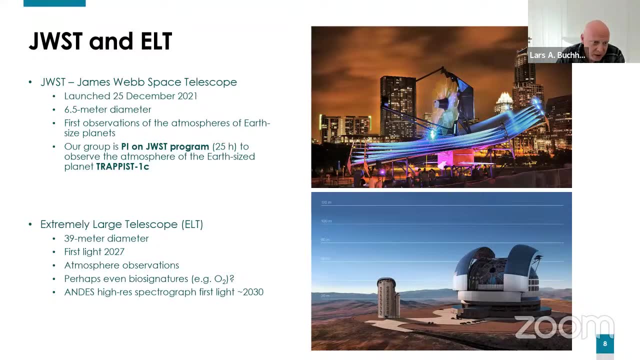 Webb. It would be excruciatingly difficult. So we have to go to these smaller red M dwarf stars in order to be able to perhaps detect atmospheres of terrestrial planets- for the foreseeable future, I think- And of course the instruments that are available to do this is the James Webb Space. 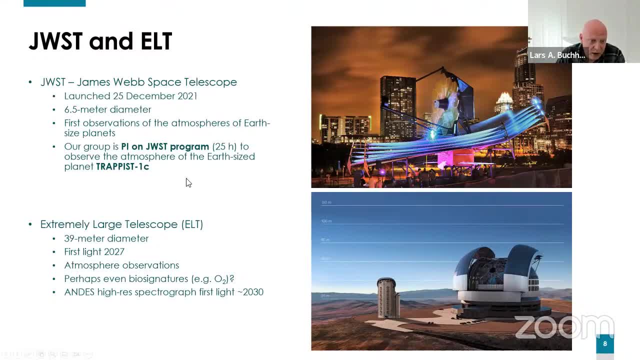 Telescope which was launched a few years ago, And we have a program on TRAPPIST-1c. I'll come back to that in the coming slides. And then there's the ELT, which has first light in the end of this. 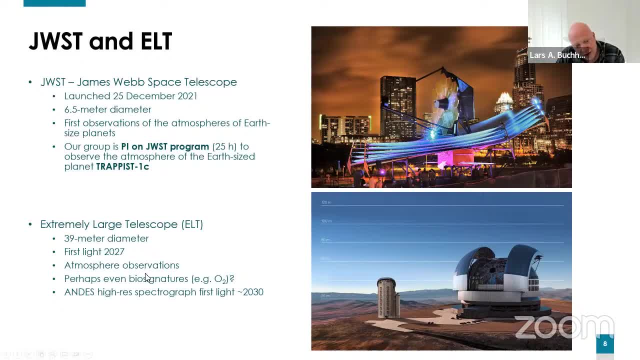 decade. And then there's a secondary instrument called ANDIS, the High Resolution Spectrograph, which is right now being planned, And the hope is that it will have first light in the early 2030s, And this will really be a workhorse for exoplanetary atmospheres, I think. 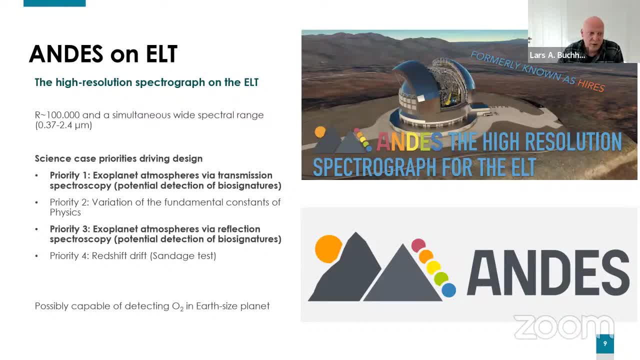 It's 100,000 resolution with a wide spectral range from 0.4 to 2.4 microns, is the envision I put the slide on just to sort of put into perspective that the science case priorities that are driving the design of this instrument. there are four different areas And two of those. 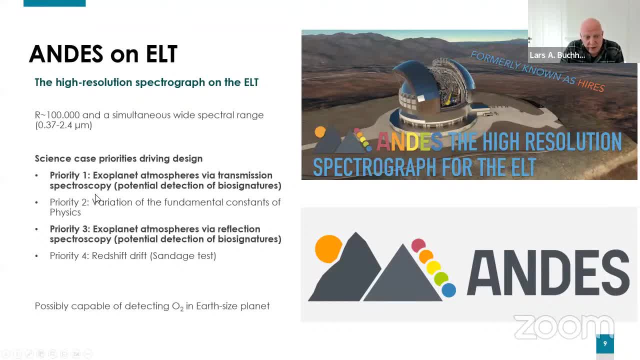 are exoplanetary atmospheres: one via transmission spectroscopy and the potential for detection of biosignatures, and then via reflection spectroscopy, which is going to be even very difficult as well. But the point is here that two of the four main science drivers for the 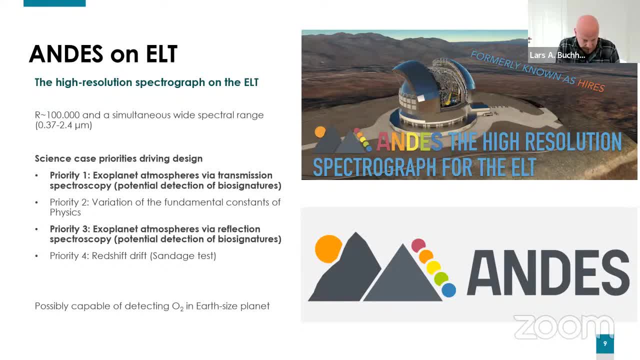 ANDIS is basically exoplanetary atmospheres, So that's going to be exciting. What ANDIS will be able to do remains to be seen. It's still under design and they're still talking about the actual how ANDIS will come to be and the funding as well, which is difficult. 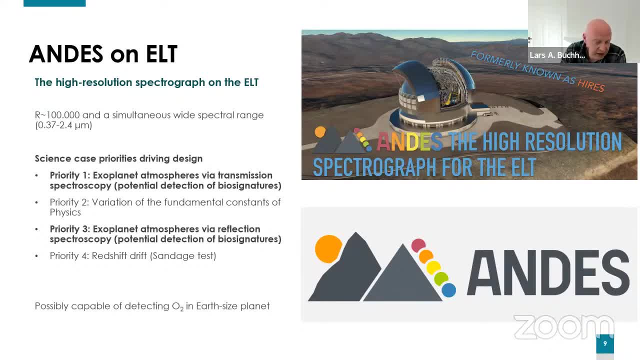 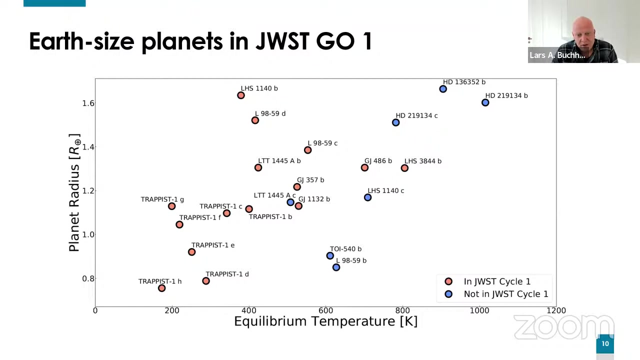 As you know, ANDIS is no longer funded as part of the ELT. It's a second generation instrument that the people behind ELT will have to get funding, national funding to fund. So that also remains to be seen if that pans out. So, turning to JWST, here's a plot of the small planets and their 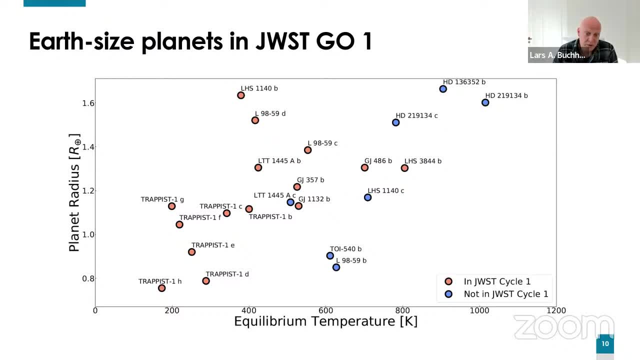 equilibrium temperature of the ones that are scheduled for observations in cycle one. So there's actually quite a few terrestrial-sized planets That would be observed with JWST. Now that doesn't mean that these will all result in detections of the atmospheres. There are various programs, Some are guest observer programs and 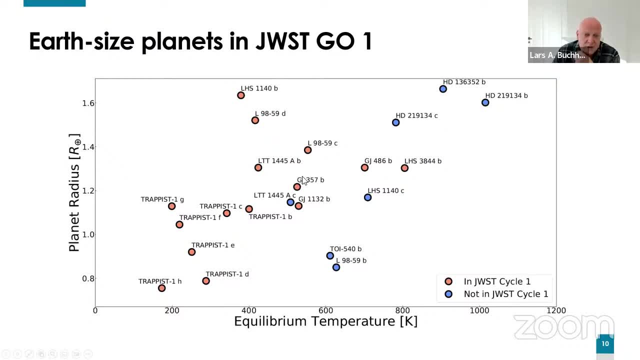 some are most of them. many of them are GTO programs in fact, And so there will in some cases be a few transits available in one of these, And here's TRAPPIST-1c, which we have a program. 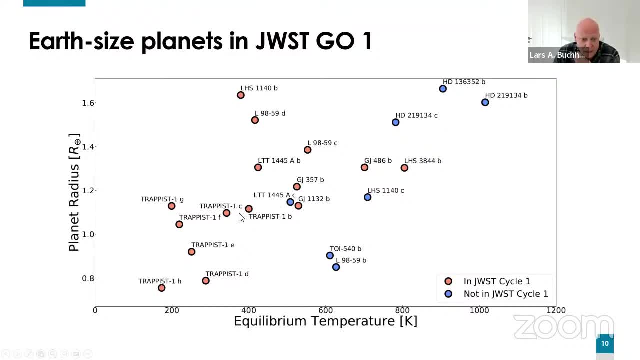 on. My PhD student, Alexander Radtke, is leading, And then what you notice, though, is that when you go to the sort of the temperate small planets, they're not going to be able to get to the transits. They're completely dominated by this wonderful TRAPPIST-1 system down here. All these 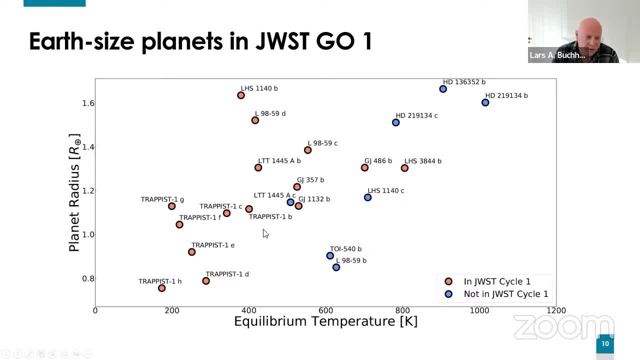 points say TRAPPIST-1.. And that's because really, TRAPPIST- as you've probably heard many, many times, is really a unique system in terms of transmission spectroscopy metrics that we can expect if the planets, of course, have atmospheres, But just from a detection. 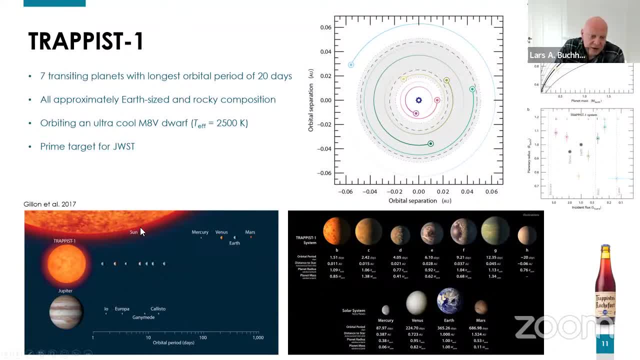 perspective. TRAPPIST is really the unique system of these seven transiting planets, and the number of them, depending on how you define the habitability, is going to be very, very high, And so we're going to be looking at a very, very short. 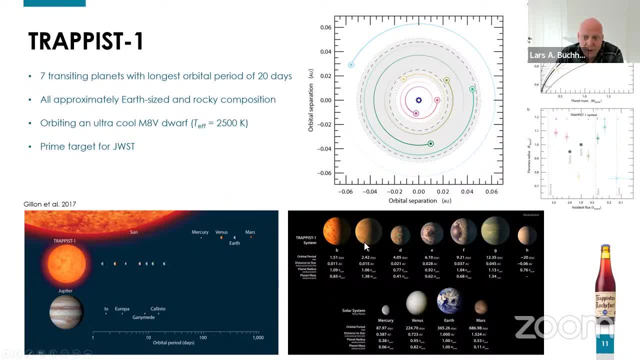 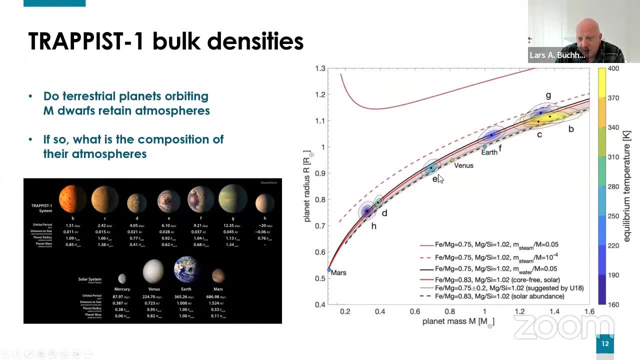 orbital period of 2.4 days And it's quite warm. It's not in the habitable zone And the TRAPPIST planets have sort of densities that are compatible with Earth-like composition. And this is from Eric Hegel's paper from 2021.. And the masses here are from transit timing. 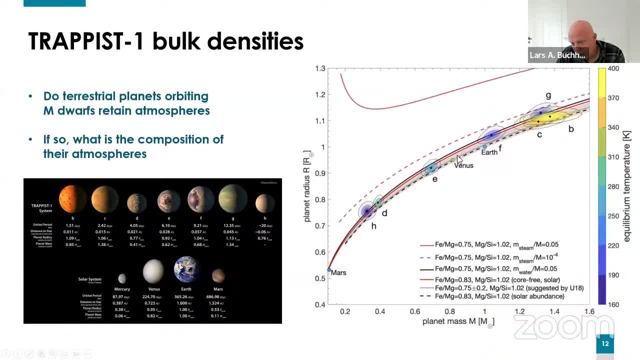 variations, And if you look at those uncertainties, they're compatible with rocky planets with atmospheric atmospheres, But they also seem to be slightly more puffy than the Earth-sized planets. Of course there's large uncertainties here still, But that could either be because of 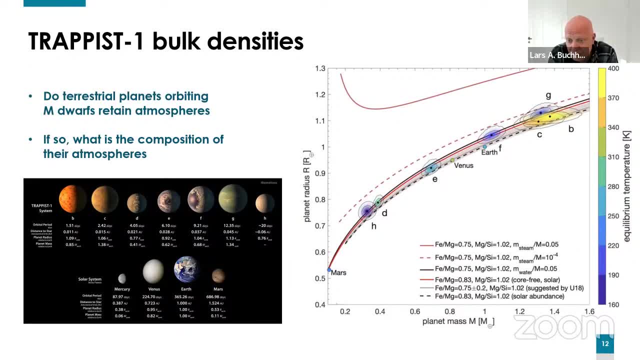 some volatiles in an atmosphere, or it could be because of the composition of the interior of the planets, or it could be because of the measurements, of course, and the uncertainties in deriving masses. This is not really velocity. The system is far too faint to do our refo. 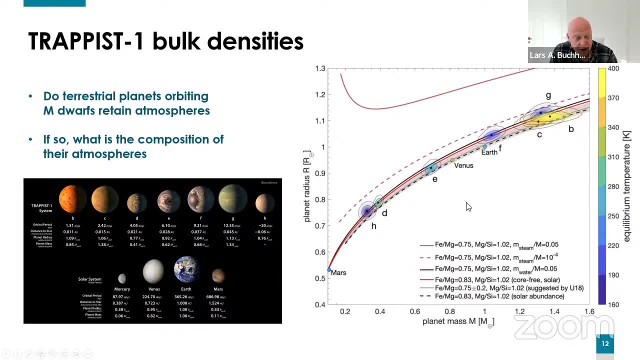 up and get masses of this type of precision for this type of star, I think the V is like 18th magnitude in V, And it's very, very difficult to get precise velocities. So the question then is: do any of these planets have atmospheres, And if they do, what is their composition? 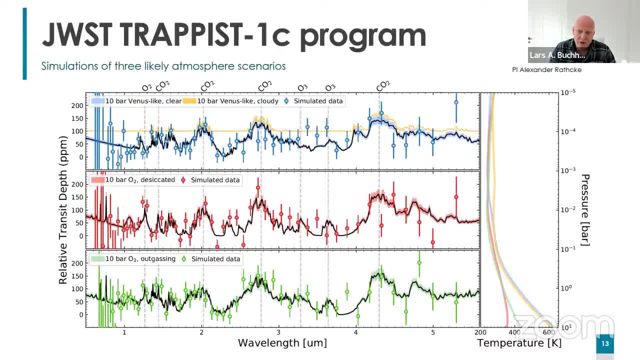 So we put in a proposal led by, as I said, my PhD student Alexander, who's now at the CFA for a year And he's returning to our group in the fall as a postdoc, where he got his own, which is great. So we put in this program- and this is from our proposal- to try to observe the 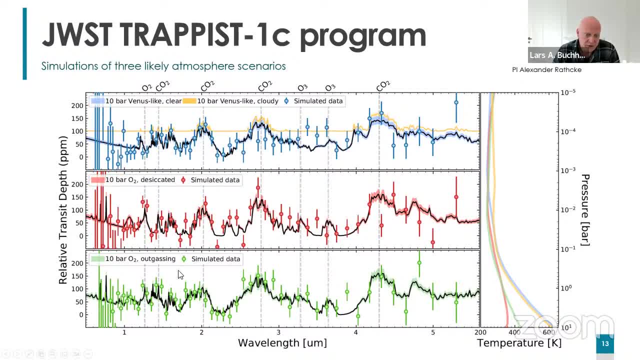 atmosphere of TRAPPIST-1c, And these are three different atmosphere compositions that we looked at And then we simulated whether we could detect the atmospheres of these planets. So the first on the top here is a 10-bar Venus-like atmosphere, a clear Venus-like atmosphere, And Alexander ran. 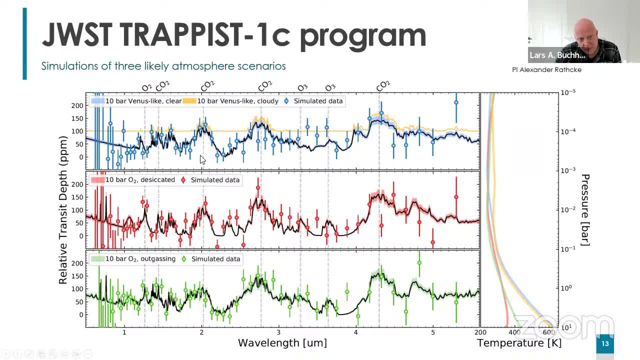 simulations on a cluster computer, simulating this hundreds of thousands of times. And this is the sort of transmission spectrum simulated from JWST, assuming four transits, And we can, with high statistical significance, detect, we simulate the CO2 features in this type of 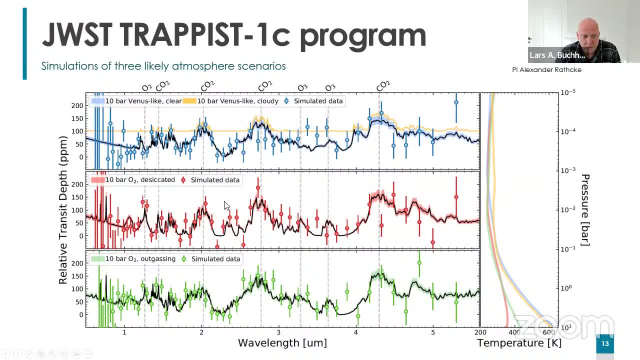 atmosphere And below there's two different oxygen dominated atmospheres. So this is a desiccated atmosphere, assuming that water has been photodissociated, the hydrogen has escaped And we now have an oxygen-rich atmosphere and we can detect CO2,. 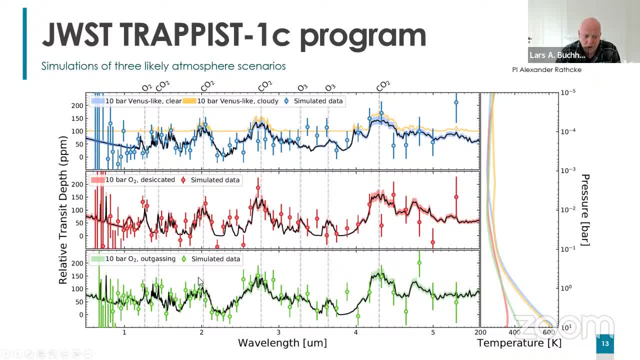 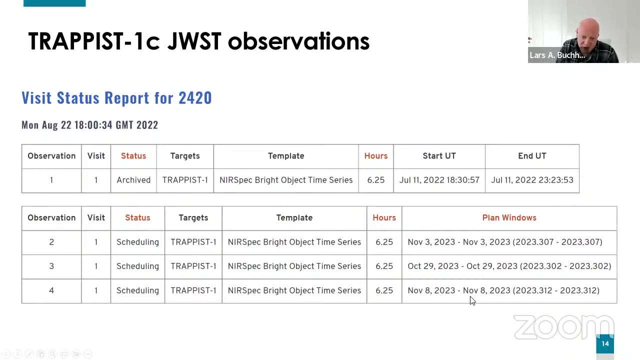 trace gases in the atmosphere, and here's a similar one where outgassing has been included to give you more co2. so this is our simulations, and then the program was scheduled sometime last year and we were. we were basically set at the very, very end of cycle one, to both our despair and relief. 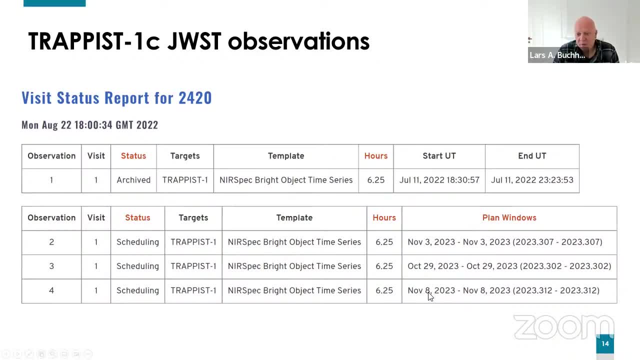 despair because it was very late, but in relief. that i mean when we had a number of months or time to build a pipeline. so we're scheduled basically to in october, november in 2023. but last summer my alexander called me on a saturday and i was like there's something up. 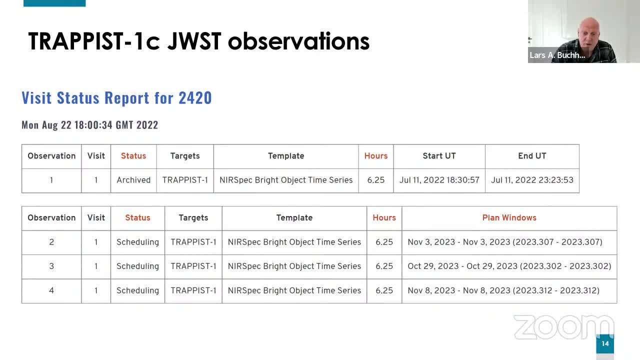 and it turns out that one of our transits were scheduled. that was scheduled very, very early. in fact, this turns out to be, i believe, the first time jwc looked at an earth-sized planet to attempt to detect the atmosphere, and so, as you say, this is in july and this was basically just before summer. 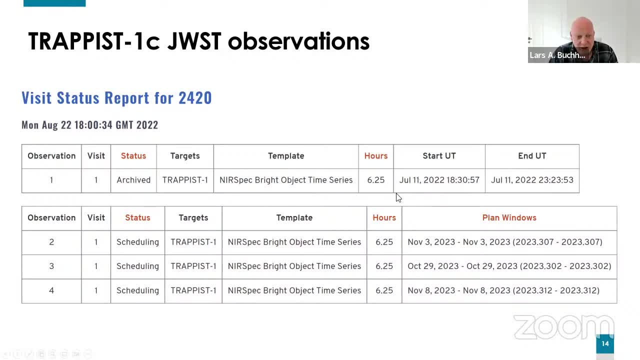 holidays and, in fact, i was downloading the data on a friday before going on vacation. so this was a bit and we hadn't really prepared any uh, any pipeline work, because we were expecting this to come in late october, uh, in november 2023. but fortunately, uh, in our collaboration, people had 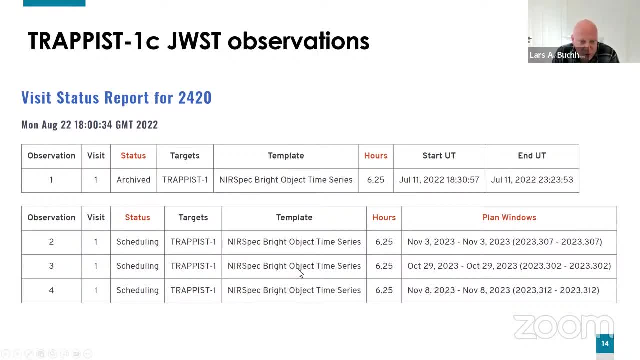 already written, some pipelines, and we had actually the opportunity to reduce the data with three different pipelines and we now have another fourth pipeline that we, alexander and i, are working on, and so here's the, here's the transit of trappist-1c and, uh, it's. it's a beautiful light curve, i think. if 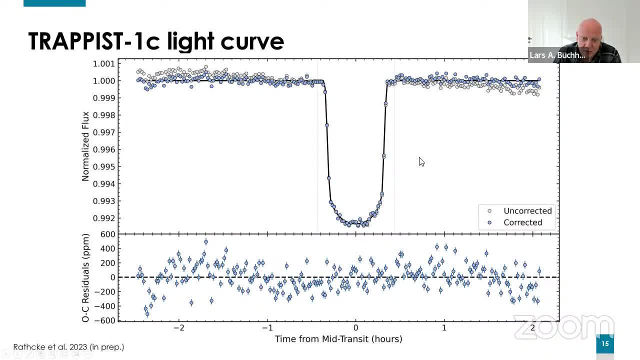 you have been in the game for some time. this almost looks like a hot jupiter back in the day. what we would expect, uh, but this is actually a terrestrial planet, of course, transiting a very small star, but the data quality is just amazing. there's some slope that we're not quite sure. 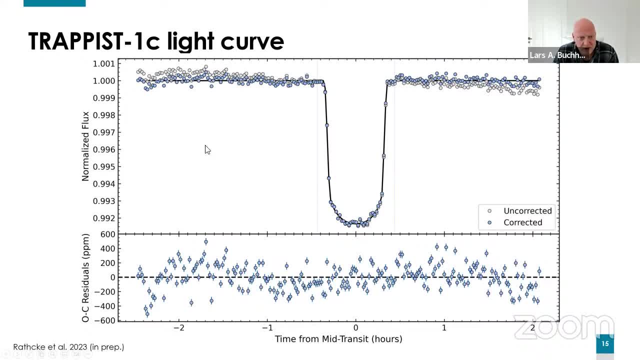 what we're reading. what type of data is? uh, we're not quite sure what we're reading. uh, there's some. uh, there's some slow. uh, there's some slow. uh, that we're not quite sure what we're reading. uh, what, the what, the origin of that is? 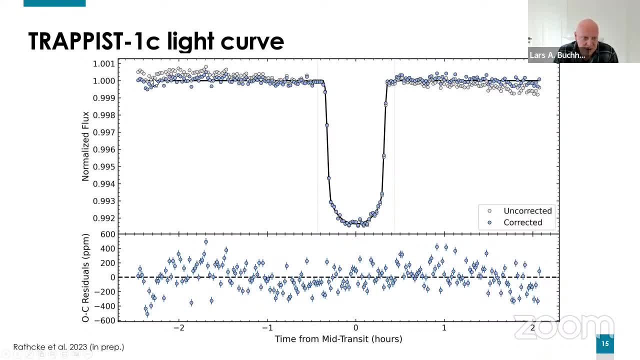 And there's still some work here on the reduction. You can maybe, if you squint, see some correlated noise in the residuals here, But this is a work in progress. This is unpublished data. We hope to publish this transit before the. 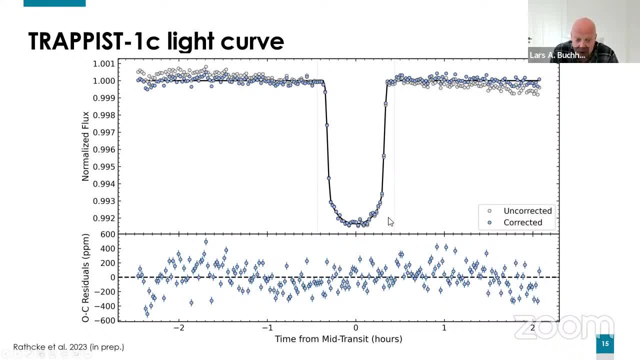 or this data before the remaining three transits And, of course, with this one single transit, we don't expect to be able to see any atmospheric features with the signal-to-noise that we had simulated. We really need the full four transits. 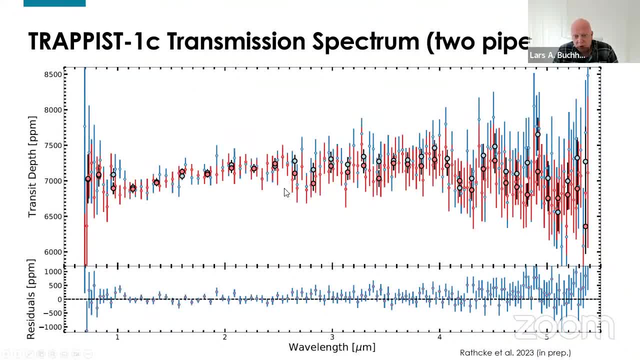 And lo and behold, we see a very flat transmission spectrum of TRAPPIST-1c And we're not able to discern any atmospheric features. of course, and we didn't expect to, The signal-to-noise we simulated was way below three sigma that we expected here. 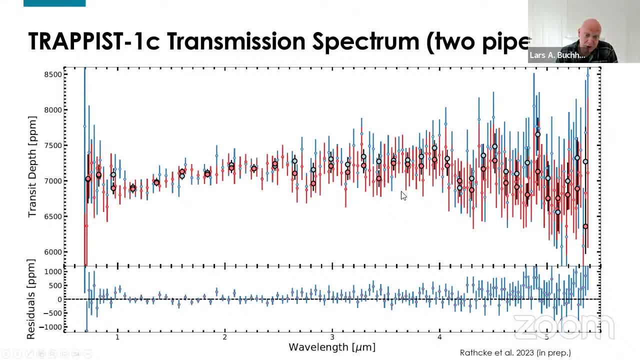 But the upside is that the signal-to-noise and the quality of the data that we're achieving is actually better than the exposure time calculator predicted. So we're not able to see any atmospheric features. So, in other words, if the planet has an atmosphere like we've simulated, 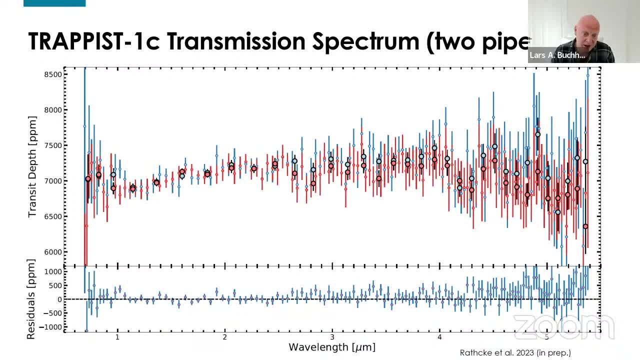 and we're able to deal with stellar activity and systematics and the planet actually has an atmosphere, then we should be able to detect it with these four transits. Of course there's many caveats and ifs there, but at least JWST and the data that we're getting. 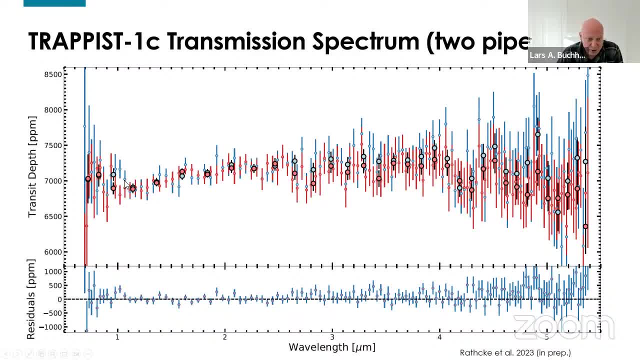 is really performing very well And there's this slope going on. You may be able to see here in the blue that I'll come back to in a minute- which we're kind of uncertain on the origin of that. But to compare, to compare with already existing data. 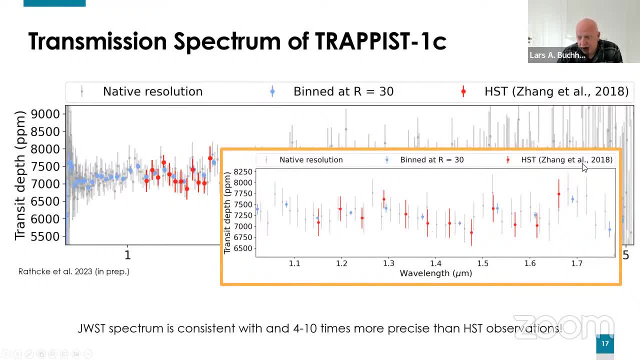 we looked at data from HST, from Zhang et al, in 2018.. And that's the red data point. I believe It's from memory. I think this is about two transits, Comparing that to the blue data points. 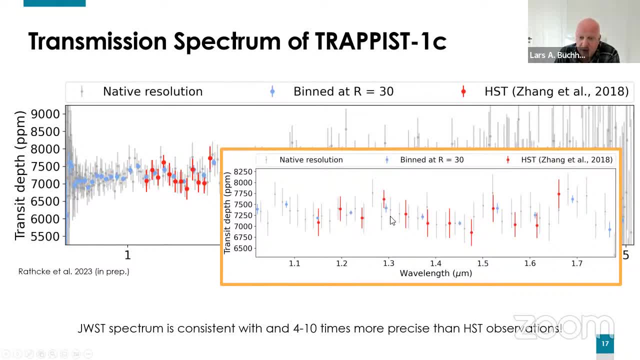 which is our data: one single transit of TRAPPIST-1c And you can see the uncertainty in the error bars and the blue data points from James Webb are highly much, much better than what came out from HST from these two transits. 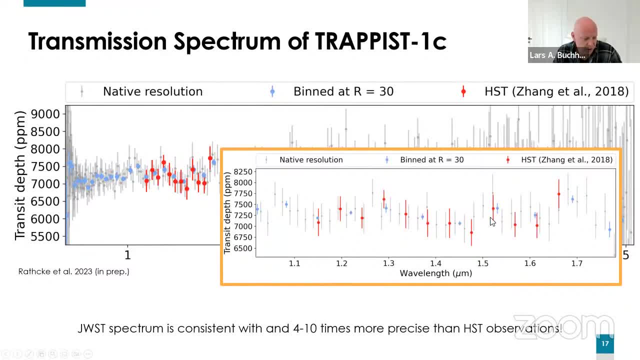 So the data quality is amazing, And I hope that some of these planets have atmospheres so we can actually characterize them in the coming years. I think we're in for some excitement there, And just to sort of give you a sense of the features that we're looking for, 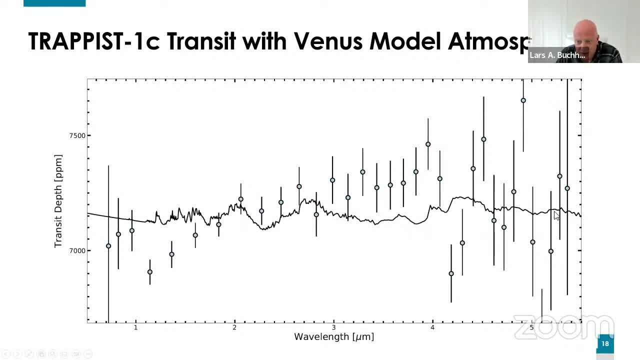 this is the CO2-dominated 10-bar Venus atmosphere that I just over-plotted on the data, And you can see that we are not able at this stage to be able to detect any of these quite small features with the precision that we're achieving. 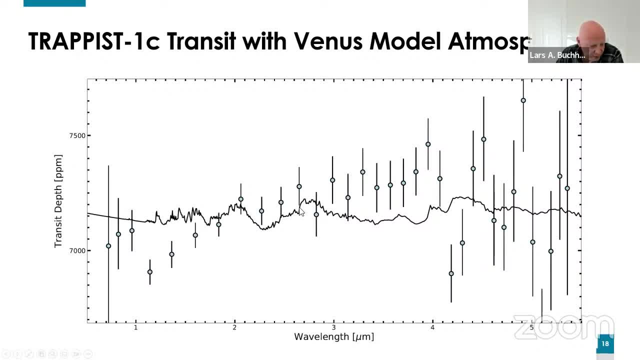 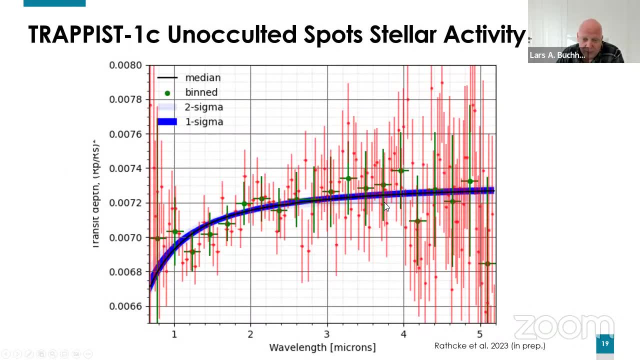 with the data. So we're not able to detect any of these quite small features with the single transit. Now, this slope in the blue, we're a bit well, that could indicate, of course, stellar activity. So we tried to model this. 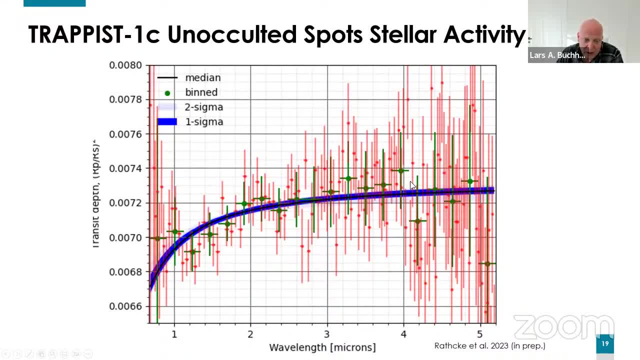 with basically a very, very simple spot model And you can sort of get this slope in the blue. And then, of course, there's some very large uncertainties. in the very, very blue part of the spectrum, Actually, it may seem like it's turning up again. 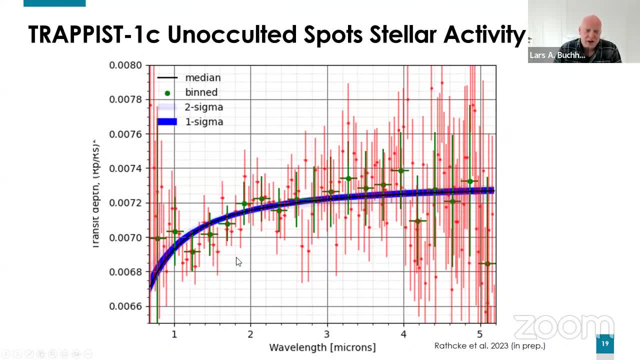 like it has a peak, And then you would have to make some sort of more complicated model with cold and hot spots. But we are able to simulate this with stellar activity, if that is what we're seeing, Because then we kind of looked at the data. 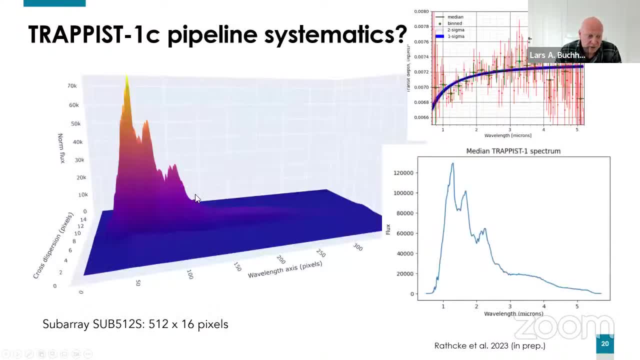 in a little more detail, And this is a plot of our subarray. It's the sub-512S, So it's the smallest subarray you can get with near-spec prism, So it's only 16 pixels in the cross-dispersion direction. 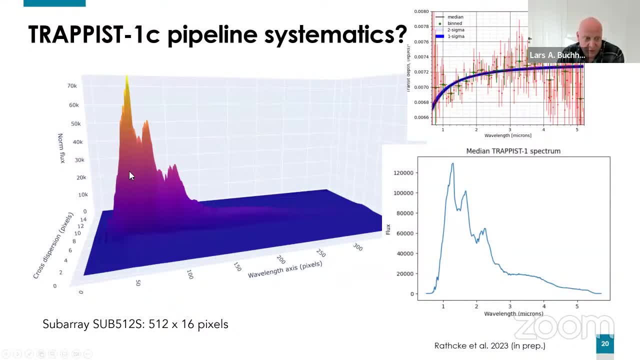 So this is the spectrum. the spectrum of the star trap is one, And you can see that it peaks very strongly here in the beginning of blue. And if you actually look at the resulting median spectrum of all the integrations, this is what it looks like. 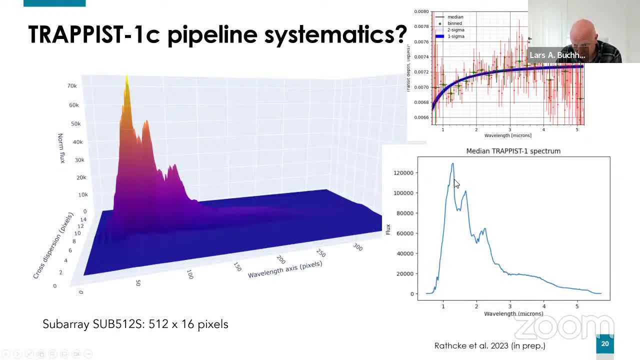 And what we're a bit suspicious about is that if I draw a line here- I tried to line these two up- the peak of the spectrum basically corresponds to the slope that dips and sort of the bottom of the slope. So this is where the peak of the spectrum is. 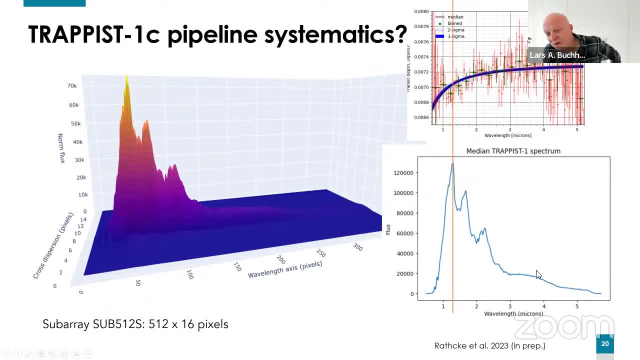 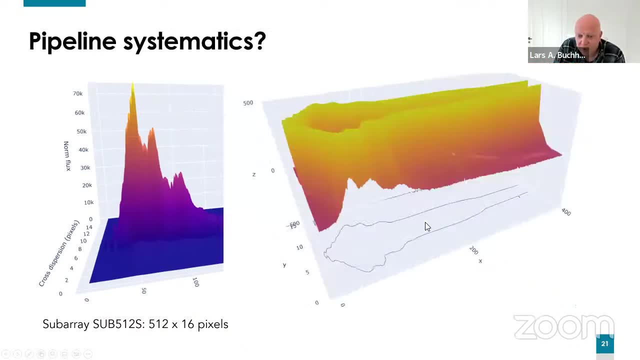 And then that slope kind of corresponds to the flux of the star. And we at least discovered in one of the pipelines some issues because we were trying to remove the 1 over f noise by subtracting the pixels that were on the edges of these orders. 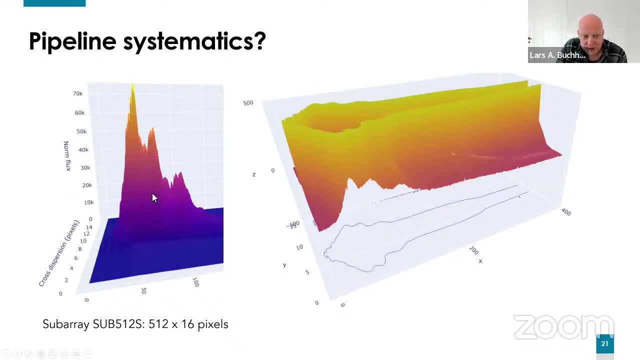 But this is a zoom in of this 3D representation of the host star And I made some very strong cuts here in order to show you that actually we're cutting off because of the small size of the subarray. we're actually cutting off the flux. 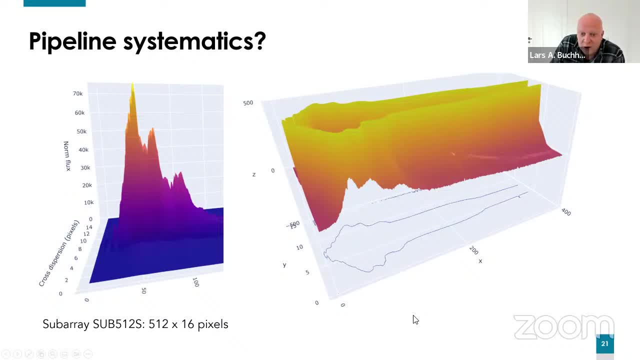 and it's bleeding out into the pixels that we're not actually recovering. And the reason we chose this was, of course, because of duty cycle, to make a very fast readout on this small subarray, And we didn't want to saturate the instrument as well. 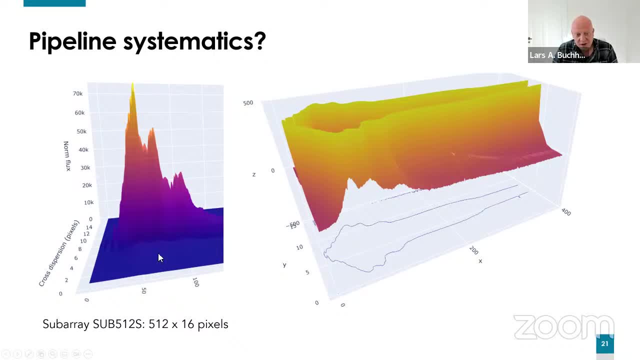 So we wanted fast readout in order to get a high duty cycle, But perhaps this subarray is actually a bit too narrow. There's another one called 512, without the S, which is in fact 32 pixels, So we may want to change mode for the remaining. 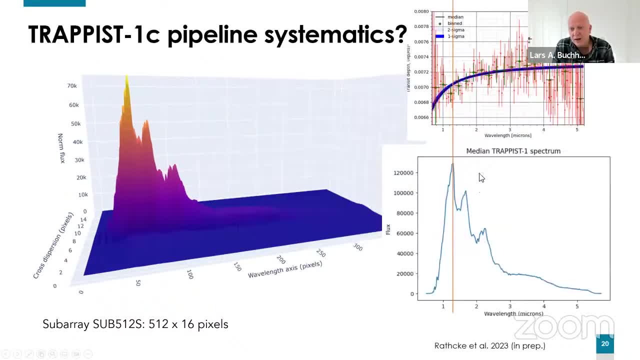 three transits that we have And we're kind of a little bit suspicious again of whether we're seeing instrumental systematics or we're actually seeing stellar activity. So that's still something we're investigating. Okay, so for the last 10 minutes of my talk, 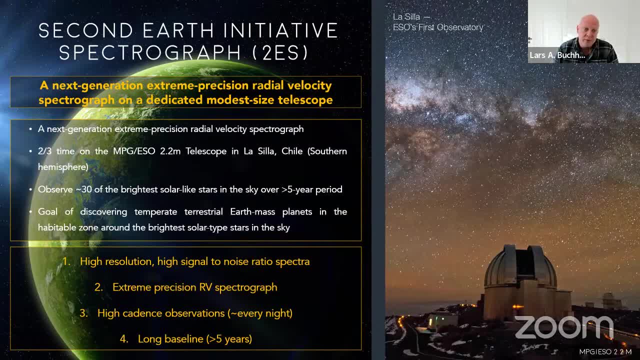 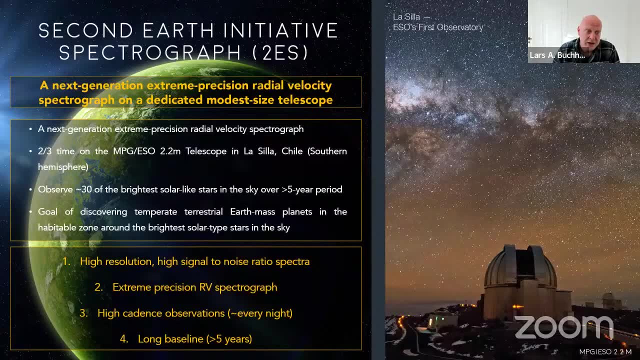 I'm going to go back to the lab. I'm going to go back to the lab. I want to talk about another project we're involved with, which is what we call the Second Earth Initiative Spectrograph, or 2ES. So the idea here is that we want to build. 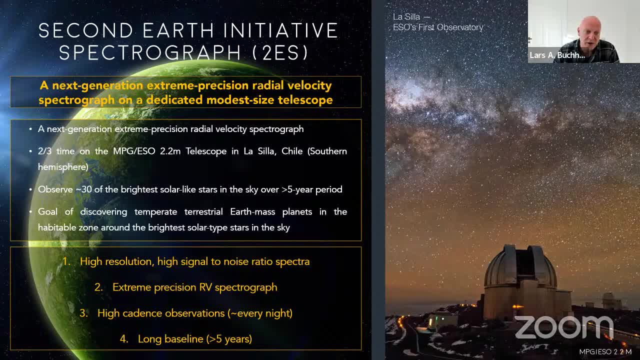 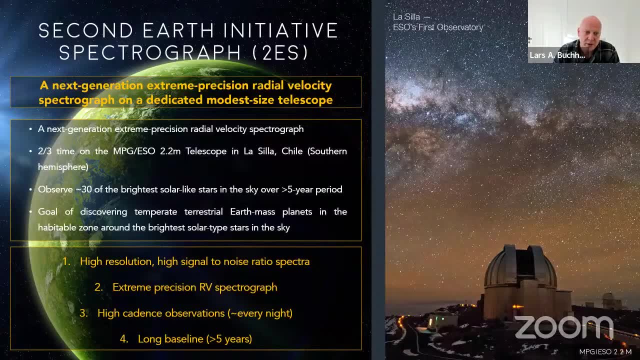 a next generation extreme precision radio velocity spectrograph and put it on a modest size telescope, but a telescope that's really dedicated to this project, basically trying to detect small planets or being solar type stars. So we're building this next generation extreme precision. 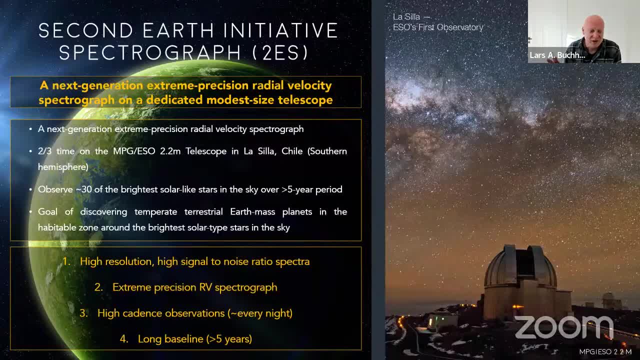 but we're also trying to build a next generation extreme precision RV spectrograph, building on the sort of knowledge that has developed in the field. There's these new fantastic instruments like ESPRESSO and NUID and EXPRESS that are these next generation instruments- RUNEX as well. 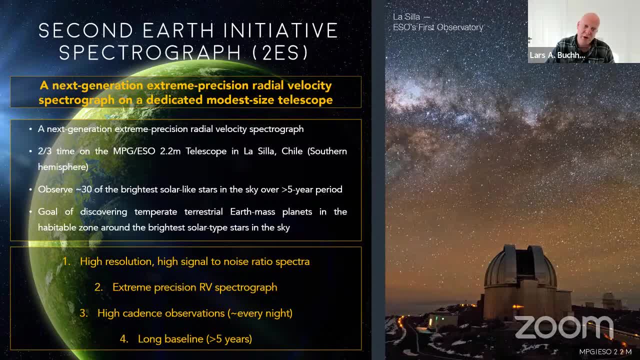 but are on telescopes where it's more difficult to make this high cadence observations of the same targets, And the idea is that we secured a two thirds of the time on this Max Planck ESO 2.2 meter telescope and the SIA in the Southern hemisphere. 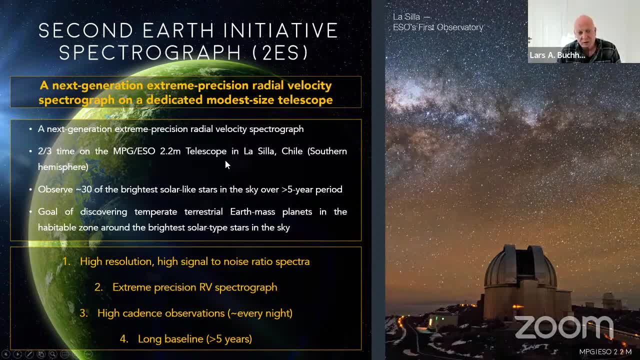 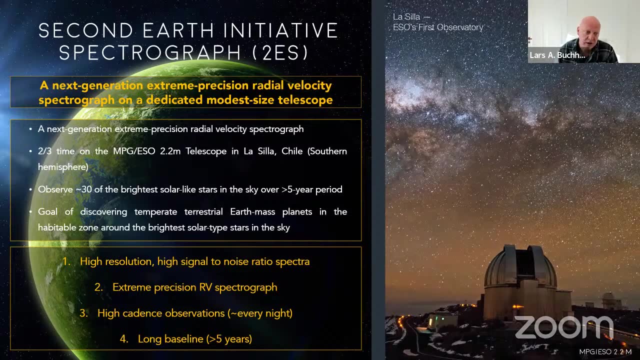 And the program we want to try to carry out is observe a couple of dozens, say 30, of the brightest solar type stars in the sky and keep pounding away on these targets over a five year period and observe them basically every single night, weather and visibility permitting, of course. 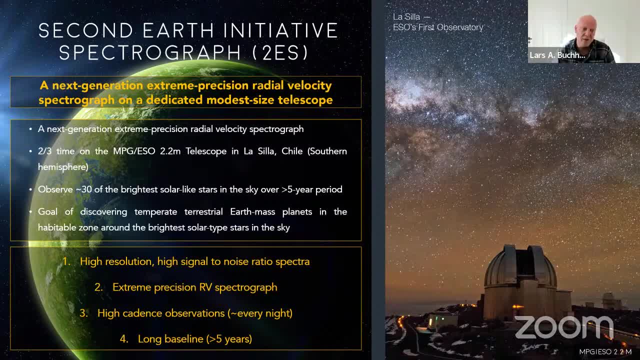 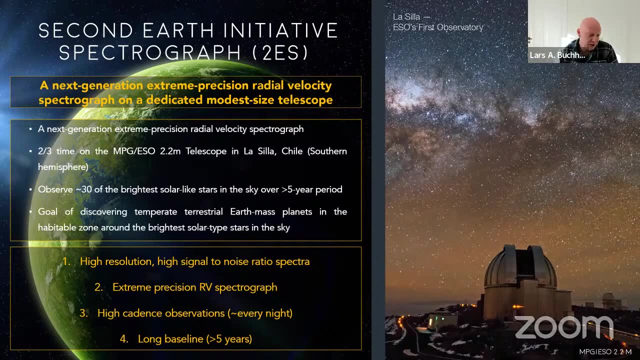 And so the ambitious goal is to try to discover tempered terrestrial Earth, mass planets in the habitable zone of the brightest solar type stars. And of course that's a very, very ambitious and difficult project and goal And two of the main issues, of course. 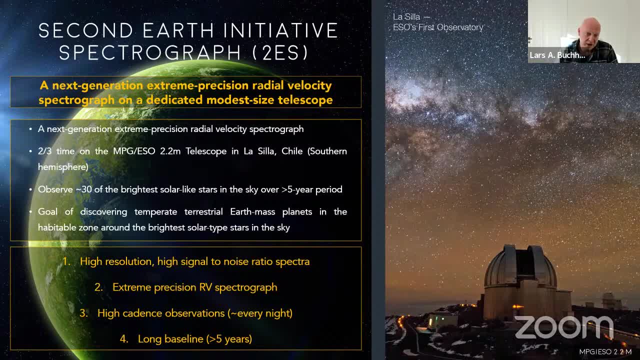 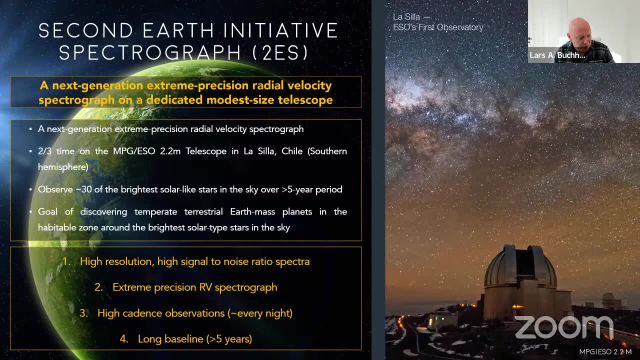 is maintaining an instrument stability of, say, 10,, 10 meter per second over years, not over weeks, And that has been. I mean, the field is really pushing towards this direction. Sometimes some people are maybe a bit overly optimistic and some are, you know, really optimistic, but you know. 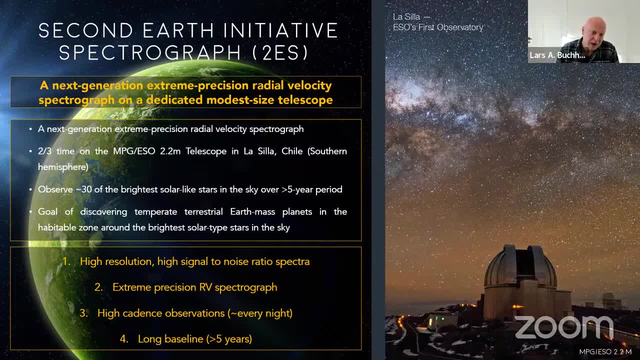 some are very pessimistic and some are, you know, so there's various, but I think we've seen data where we're looking at sort of 30, 20, 30, 40 centimeter per second precision over time, scales that are slightly longer. 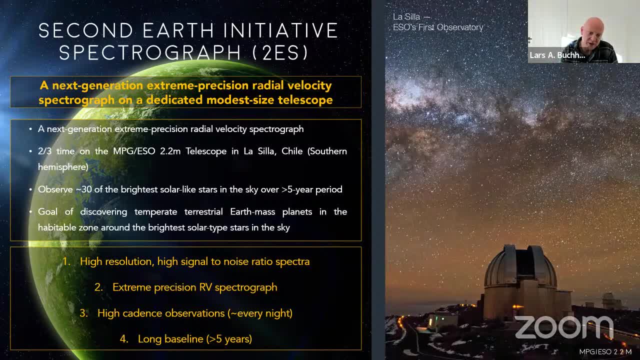 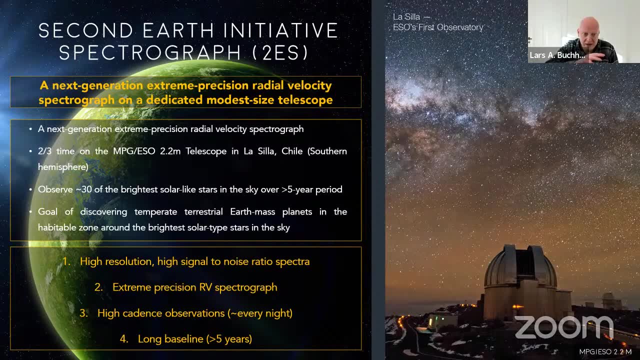 So the idea is to sort of combine four things: high resolution, high signals, noise spectra, extreme precision, radio velocities, high cadence of observations, So we can really detail the activity of these stars, and a long baseline, because one is the instrument. 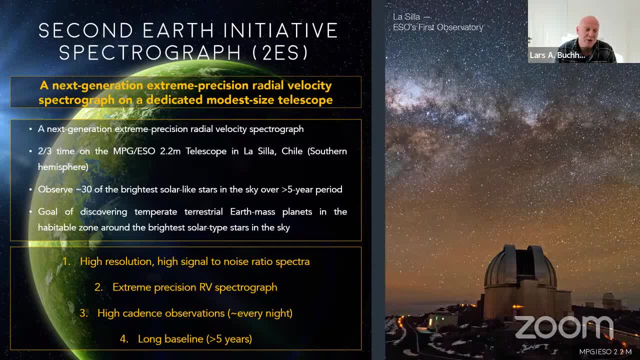 instrument stability, of course, and the other major major issue here will be the stellar activity, which is going to be a massive issue. trying to mitigate that because we know these stars will be active, even though we want to choose the brightest and most quiet solar type stars. 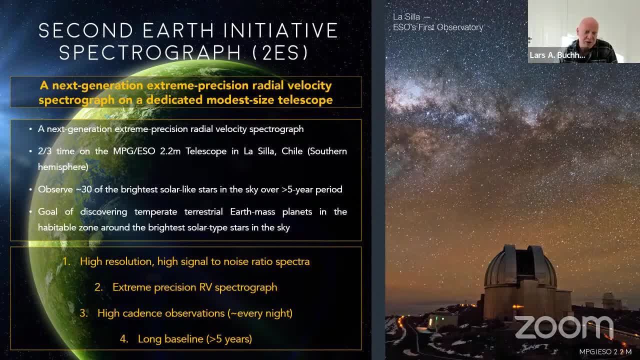 stellar activity is going to interfere And we do have to figure out how to mitigate stellar activity down to that level, which is not solved and hasn't been done yet. But we believe that building a data center, building a data set like this, may allow us. 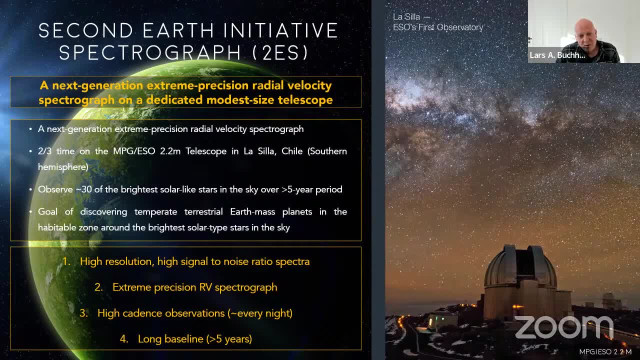 at least that's the best in our view, the best option to be able to really try to mitigate stellar activity. There's, of course, the sun, but the sun is not a very quiet star. In fact it's kind of somewhat quiet. 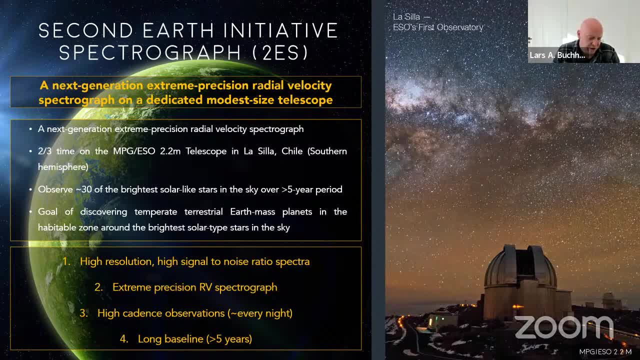 but there are other. there are stars that are better suited for this than the sun, And that's, of course, all the solar telescopes. the data is wonderful, but we don't have that kind of data for bright solar type stars, Right. 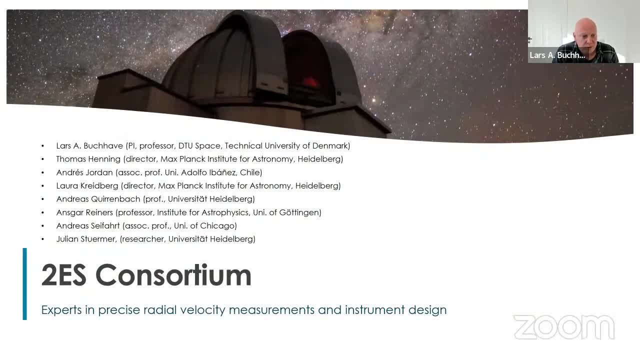 Right, Right. So those are the types of stars we want to observe with the secondary spectrograph, And the hardware of the spectrograph is now funded. We have the majority of the funding for the hardware and laser frequency comb calibration that we envision for the spectrograph. 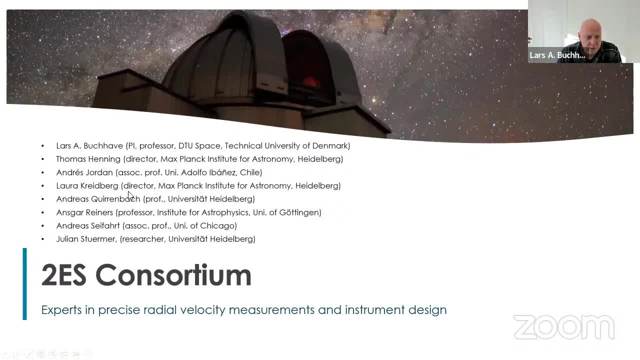 And here's sort of the consortium. I'm the PI of the project. We have Thomas Henning and Laura Kreitberg from the Max Planck Institute, Andreas Jordan, Andreas Kurenbach and Ansgar Reines From Chile and Heidelberg. 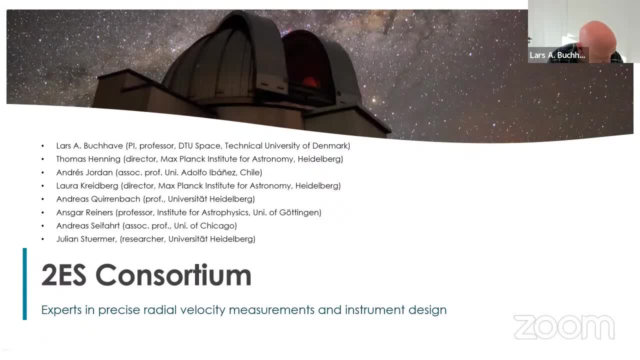 And then Andreas Seifert and Julian Sturmer, who were instrumental in building the Maroon X spectrograph, which Jacob Bean was PI on. So it's basically building on the knowledge from what went wrong, so to speak, with Maroon X or the other instrument. 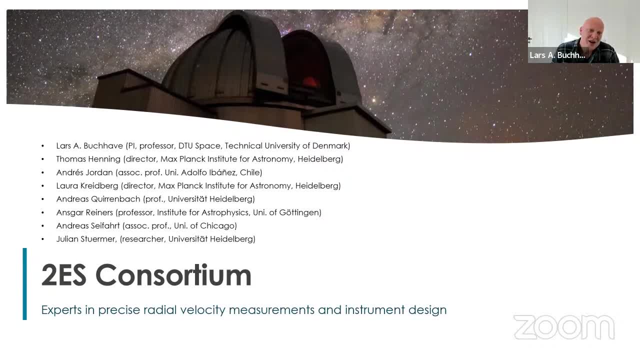 That's not the way I meant it, but building on the knowledge that we have from those instruments, because we can always try to do it as the precision as well as we can, but there's always issues that we haven't thought of. that will be the obstacle for this long-term stability. 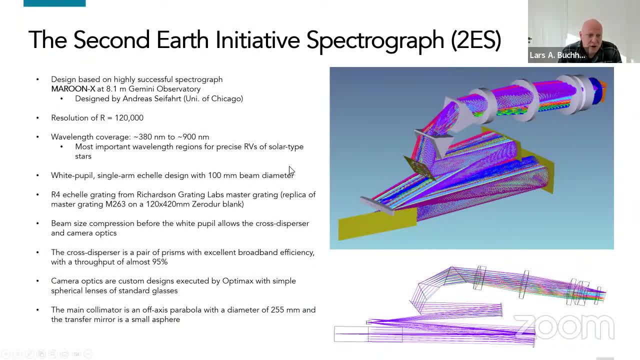 So the spectrograph is about a resolution of 120,000, like many of the other spectrographs, And it's an optical going into slightly into the infrared at 900 nanometers, And I won't go into all the gory details in this slide. 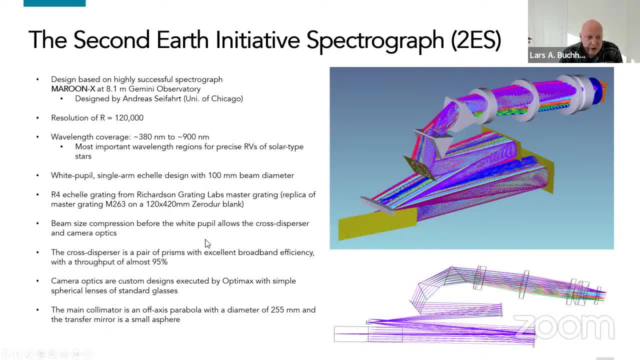 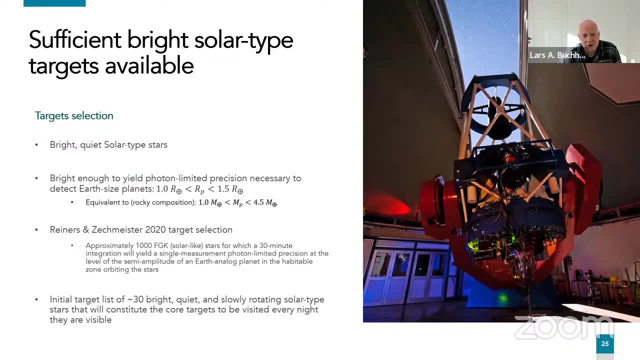 of the details. This is the spectrograph, But I do want to talk about target selection because the question is: can you, is there actually enough targets for a model size telescope like a 2.2 meter? And, if you want to look at bright photon, limited precision. 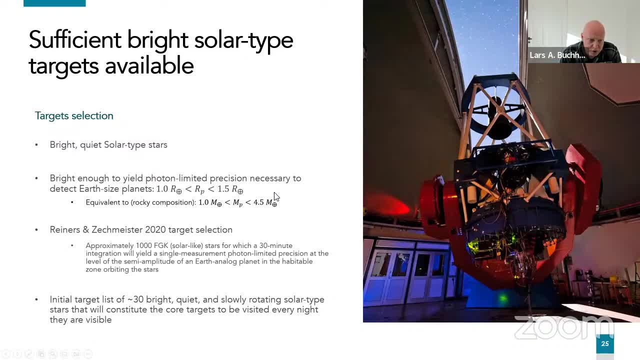 that's necessary to detect earth size planets defined as between one and one and a half earth radii. that gives us earth masses in the rocky composition between one and four and a half earth masses. Then we used and Mattias Segmeister's 2020 paper to do a target selection. 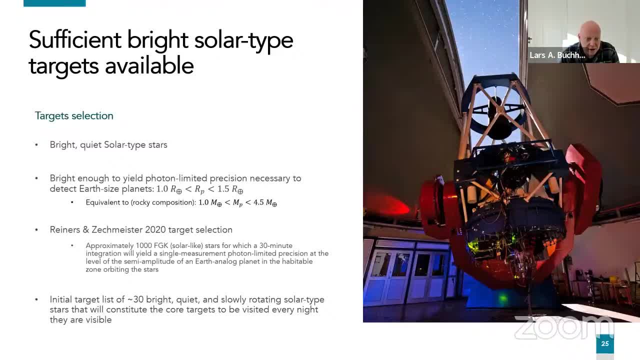 And we come to about a thousand solar-like stars, FDK stars, that we can observe, And we set sort of a maximum observation integration of 30 minutes And that will lead to a single measurement photon, limited precision at the level, that's, that will be able to detect the semi-amplitude. 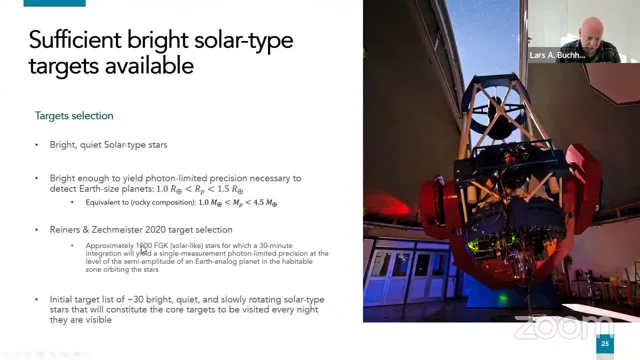 of an earth-like and an inhabitable zone. So there's there's a bunch of targets, in fact, that are bright enough, And we have worked on selecting a initial target list of 30 very bright, very quiet and slowly rotating solar type stars. 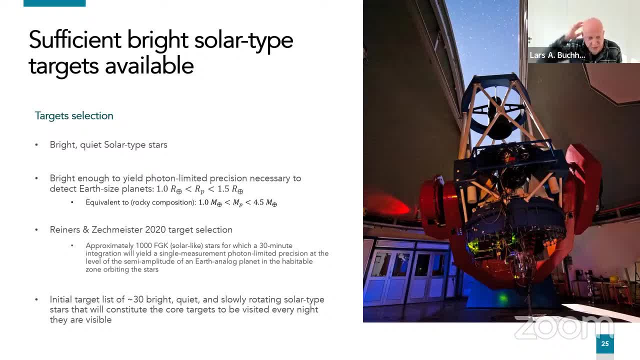 In fact we have a special proposal to go after four of these and try to make sort of a dataset that is reminiscent of what we could imagine we're getting from the secondary spectrograph, And already we were running into problems we wanted to use, especially every single night. 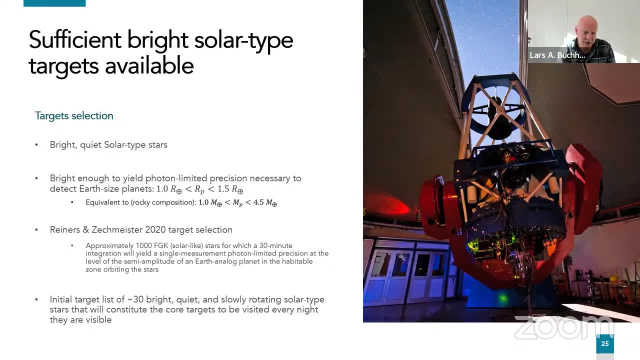 to observe these four targets that we've got time on on the special, but that's really difficult to schedule and that's kind of the point of the spectrograph that we're trying to build is to to really, uh, get a very high cadence detailed data set. and of course, there's also another project that you probably have heard. 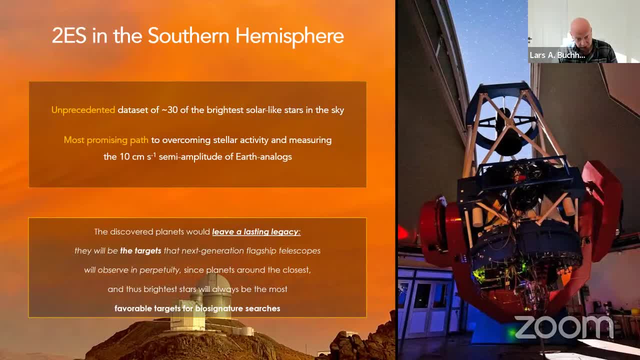 of which is arch three or the terror hunting experiment which will be, is a very similar type of spectrograph, uh, or at least the. the goals of the spectrograph are the same, which will also be on a two meter class telescope, but in the northern hemisphere, so it's very complementary to our 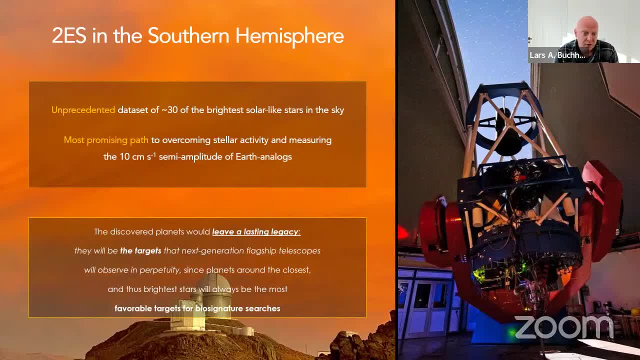 project and uh, and so the idea is, of course, if uh, radian velocities is able to do this, i i believe this is the way forward, and and we would discover planets that would really leave a legacy, a lasting legacy, because those would be the targets that are the best for next generation. upcoming space-based 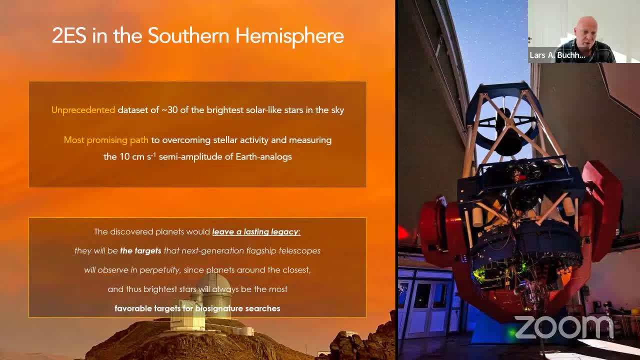 telescopes that can observe or will try to observe the atmospheres of these planets and we can sort of see when we're. i'm in the end, this uh uh working group on the, on that spectrograph, for the, for the elt, and it's really one thing is knowing the occurrence rates of planets, but actually 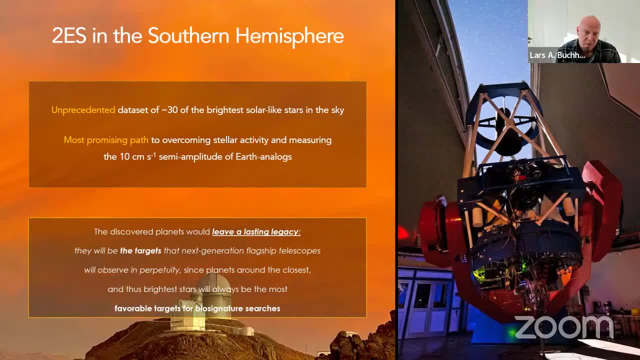 having targets to specify to, to help uh specify these next generation instruments. it's incredibly uh valuable when you're trying to figure out what signals, noise, you can achieve, and so on and so forth. so having these, these planets, would be a tremendously exciting uh for the next generation telescopes also. that. 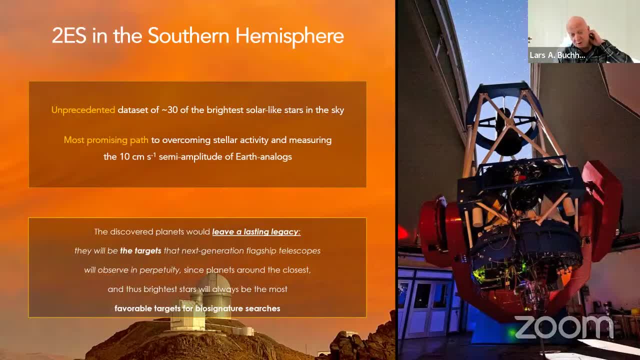 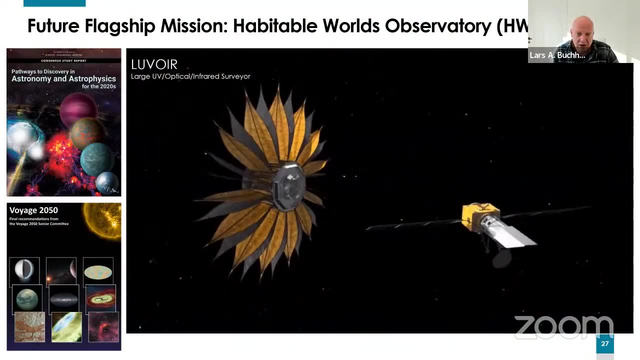 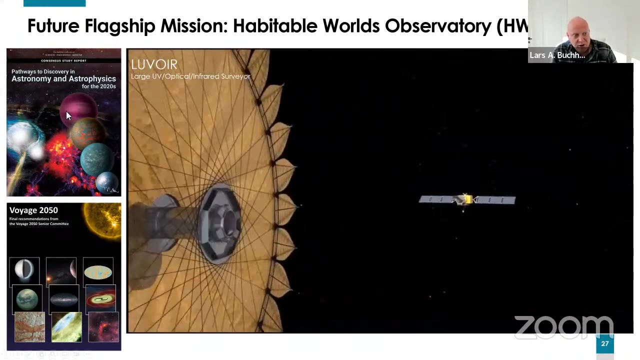 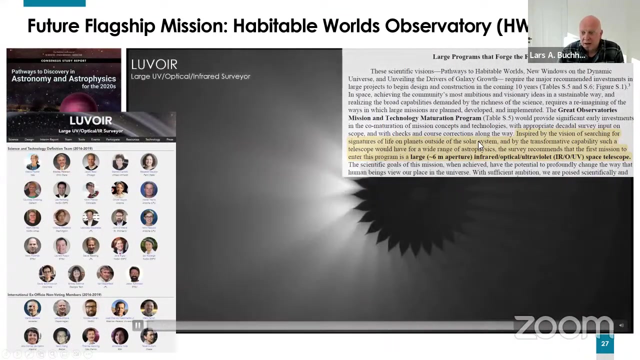 would also alleviate the need for a direct imaging survey with a very large telescope like one of these. this is from the duvar pre decadal the survey. that that, that video. but as, as you may know, or many of you probably know, the decadal survey recommended a very large uh class. 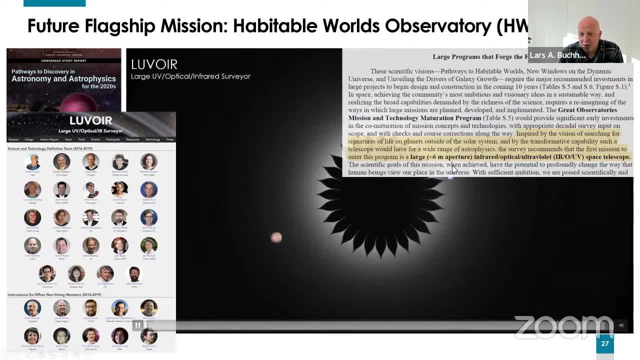 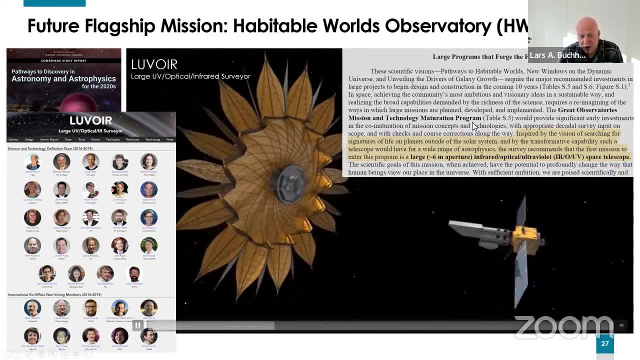 intro infrared optical ultraviolet space telescope with the goal of observing the atmospheres of terrestrial planets, and it's now, i believe, been called the habitable worlds observatory and the starting, uh, starting to go into to the planning phase. so the idea would be to try to 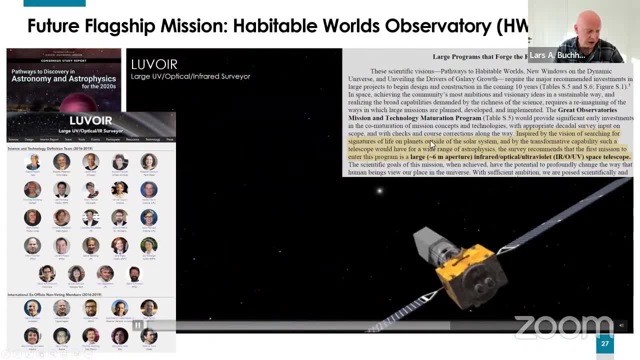 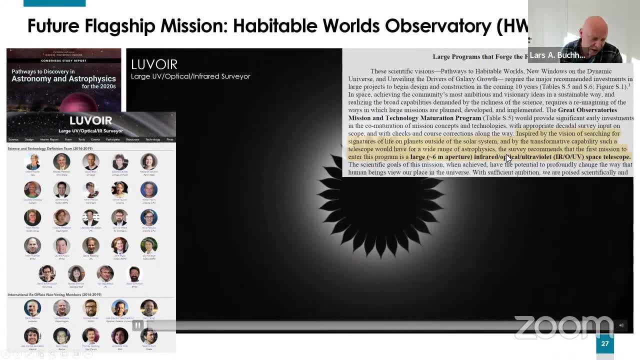 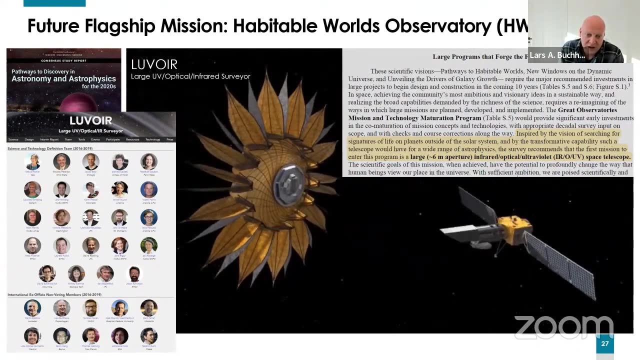 find targets, rather than uh to do sort of a direct imaging search with such a large telescope, which would be very costly and difficult. uh, if, if it's at all possible, of course i i reserve the option that we cannot uh alleviate stellar activity down to the 10 centimeter per second level. 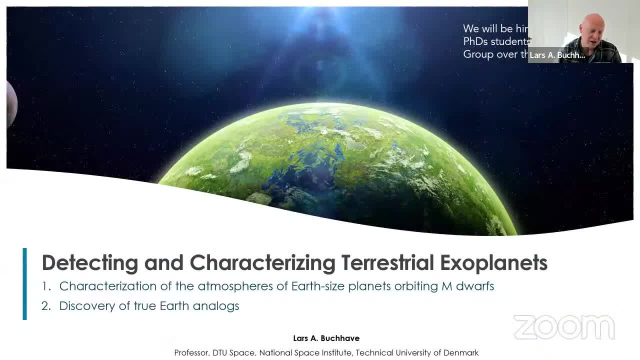 but that would also be a result, although it would be slightly disappointing. it's also it would be important to know if rvs are simply not the way to go to detect earth uh analogs in the in the around solar type stars. so with that, i want to, i want to. 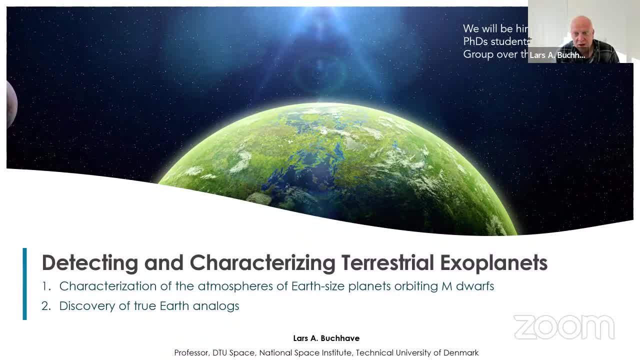 stop my talking and i'm happy to discuss and have questions. i do want to just say that we recently got a rather large grant and we're going to be hiring a number of pc students and postdocs over the next five year period. so if people that are listening are interested in this, 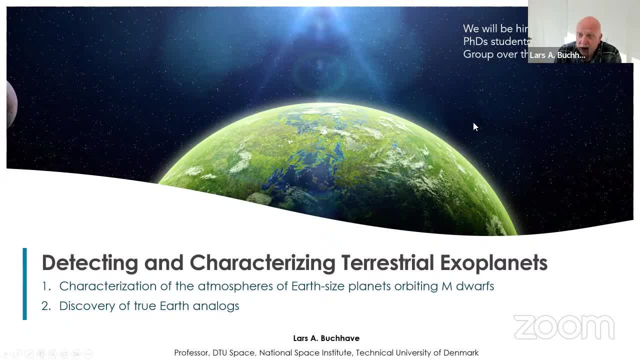 please don't hesitate to contact me or keep an eye out for uh for um, for you know calls uh for applications in our group. so thank you so much and i'm happy to talk and discuss. thank you very much, lars, that was. that was great, um. we clearly have a lot to look forward to over the next few years and 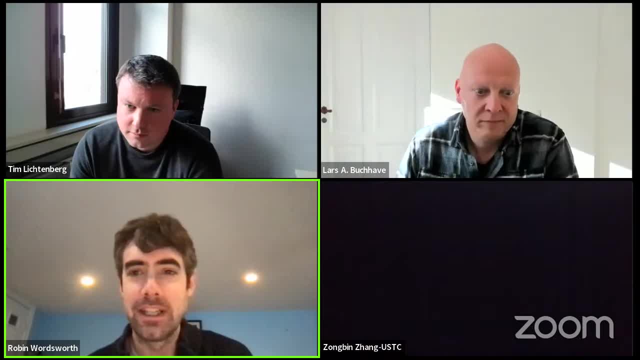 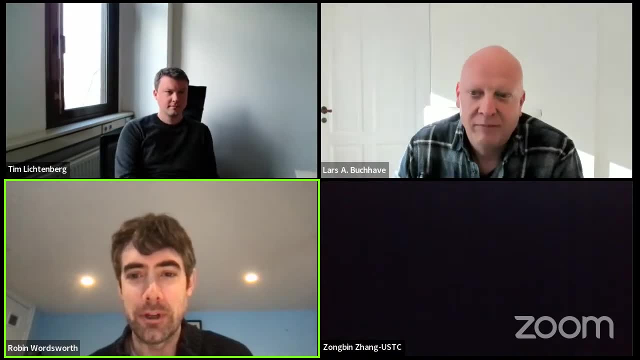 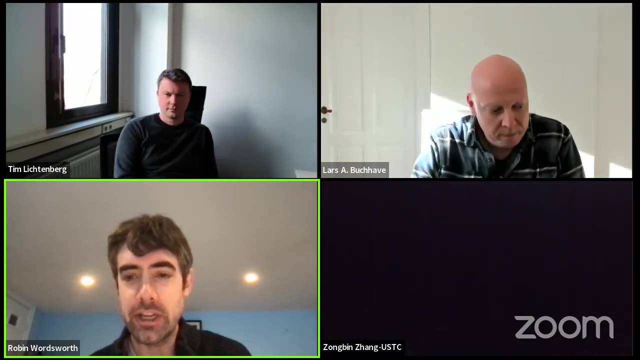 i also appreciate the the dive into um pipeline systematics. it's not. you don't always hear that in talks and it's great from a theory perspective to see some of the inner workings that goes into these things. so the floor is now open for questions. um either raise your hand or 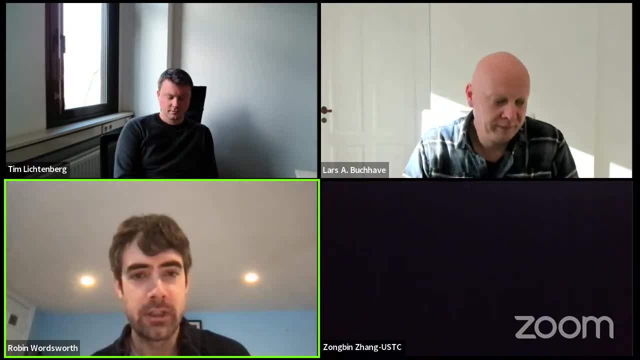 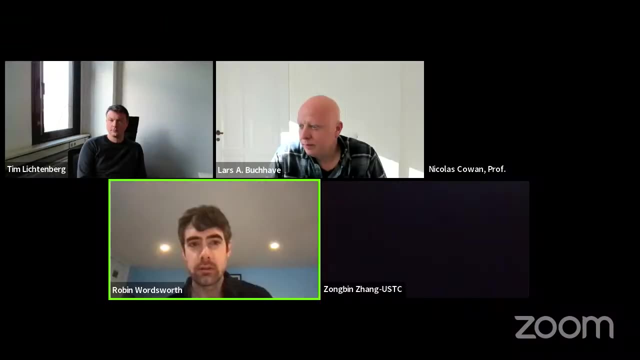 just put your question in the chat, completely up to you. so we got a question from nick cohen. go ahead, nick. yeah, so i don't know if it's a comment or question, but have you put some thought into um with this kind of- uh, search for earth-like planets? 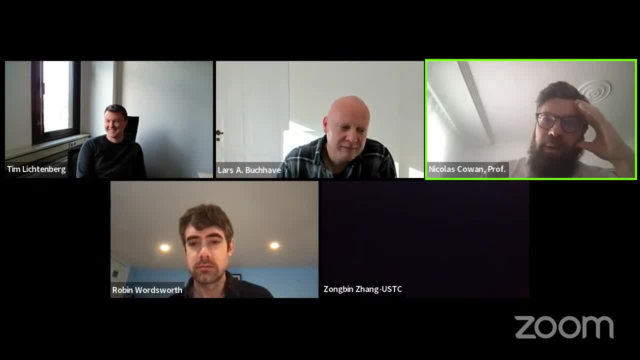 around sun-like stars. um, even if you can't actually detect true earth twins, i'm curious about particularly looking at like our planets and seeing if we can establish with some kind of more scientific evidence that some planets are more like stars than planets. um, i'm curious where so. 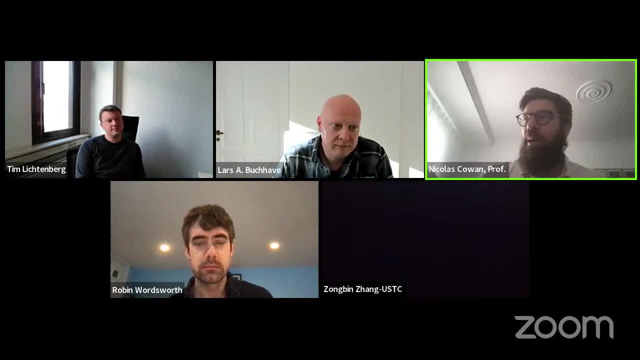 twins, just the upper limits you would get. um would still be super useful for a direct imaging mission, because when we start seeing a dot in direct imaging and reflected light we will have no idea what mass that dot is. and if we could at least rule out any like neptune or sub-neptune. 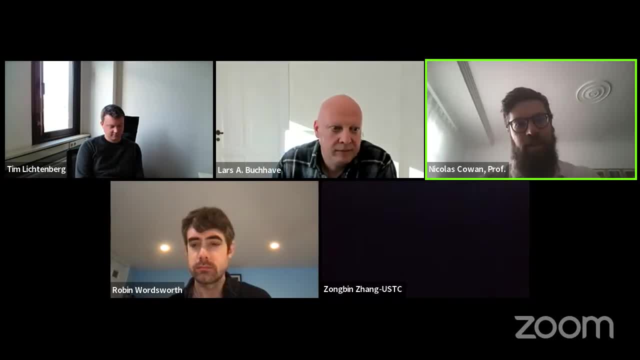 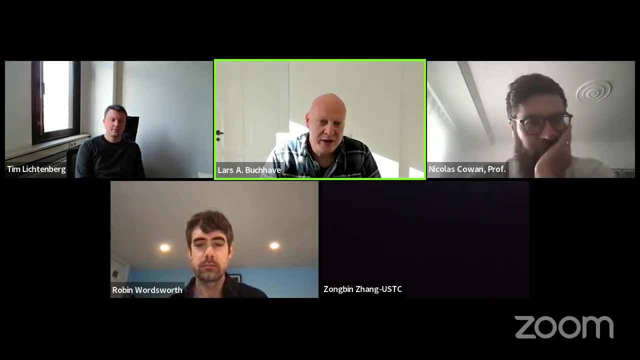 scenario, then we would at least know that we're looking at a terrestrial planet, even if it had not been detected previously with rv. yeah, true, i mean, we know this from all the transiting follow up, rv follow-up that's been going on right. it's much easier when you know there's a planet and 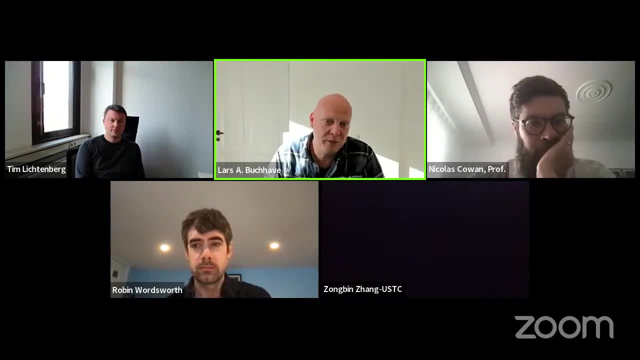 you know what to where to look than the blind rv, you know, the rocky planet searches. that also goes on, uh. so so i think, if you, as you say, detect like a, say, a dot, and you think there's maybe a planet there, uh, having that constraint and then having the rvs would actually be very, very, uh, very useful. 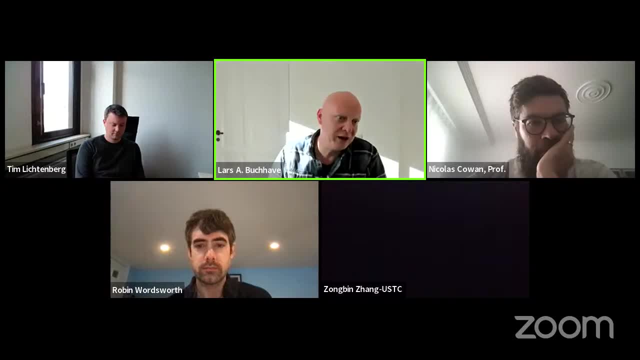 we haven't looked into the number and and we haven't estimated what what that could sort of mean in terms of of uh, of upper limits, but but it's certainly true that you know, if there is a detection from some other uh type of uh observations, like direct imaging or transits, then it's. it's actually much, much easier to to look at. 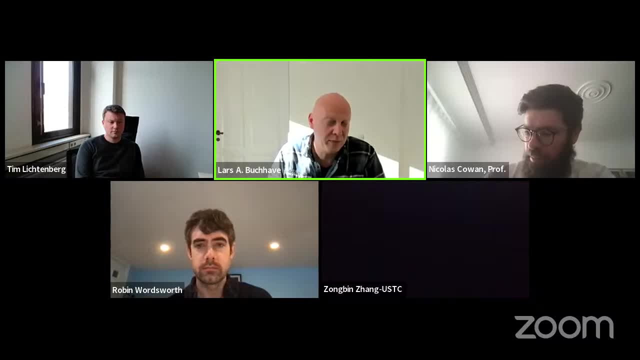 the, the radio velocities, uh, afterwards. so that's certainly something that can be done, if, if, if those targets that we're looking at, you know that that data set will be there, uh, um, once these uh direct imaging emissions might fly later in the, in a couple of decades. i don't know if that's. 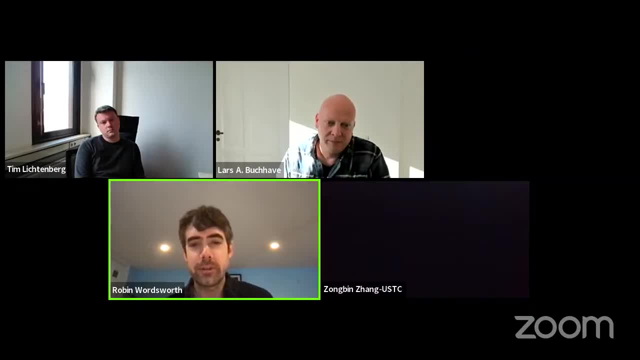 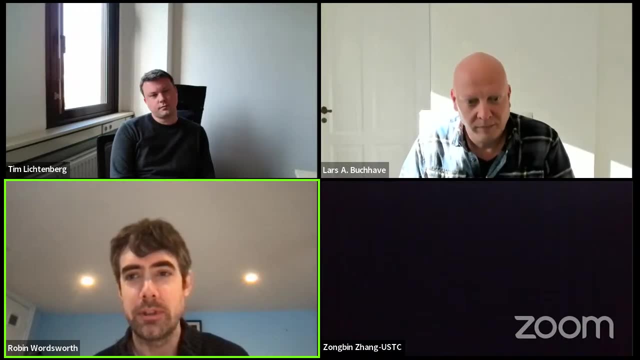 the case? i guess yeah, and i mean just to follow up on that point. i mean for good reason. earth-like planets around sun-like stars are kind of the most exciting, but there's a huge science case for other types of rockies or even up to sub-neptunes in habitable zones around sun-like stars as well. so i'm 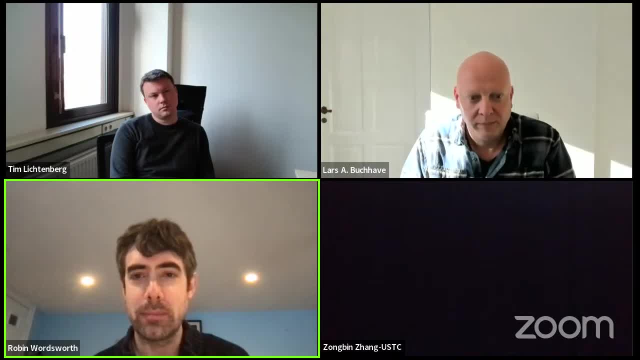 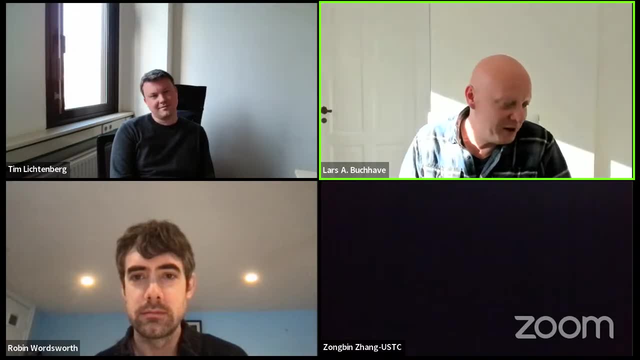 wondering for the 2es science case is that, is that part of what you're proposing. well, i mean yeah, so there's no. i mean, these terrestrial plants in the habitable zone are not going to be alone, right. so so sort of the auxiliary uh payoff would be, hopefully that we discover a number of planets in in what i expect. 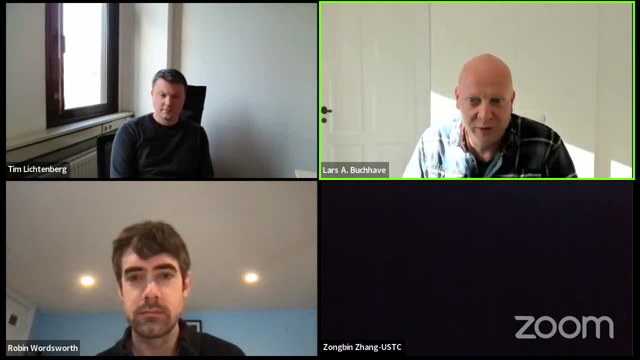 would be multi-planet systems and also, you know, tease out the masses of larger planets in these systems as sort of a side goal. but the main, the main thrust of the project is really to to make this this giant leap towards trying to detect terrestrial planets in the habitable. 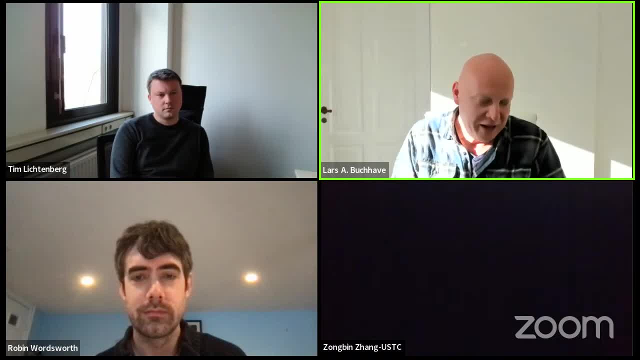 zone of solar types, which is incredibly hard and, as i say, i i i know people are skeptical and and it may be that this is simply just not possible to overcome the stellar activity at this level. uh, that, that's there, but i think this is the the best way of trying to do so, in my my view. 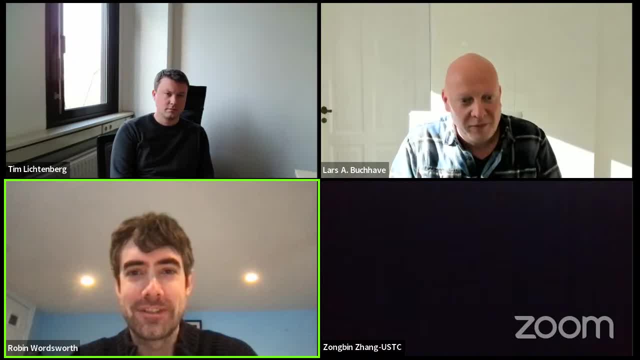 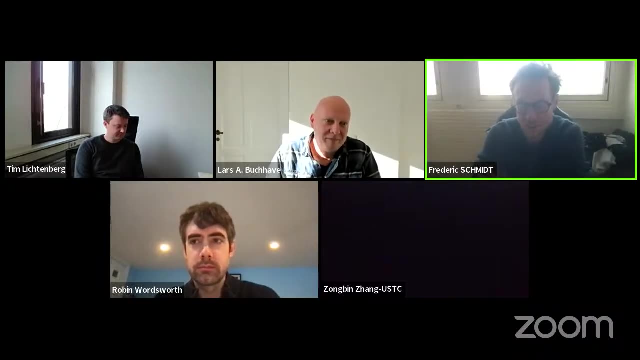 yeah, sending me to the second stability over years. it's not, not easy. that is not easy. a question from friend frederick smith: hi, very nice to thank you. maybe a naive question: is that possible to make the difference or detect a moon that could be around those planets, and especially for on the g double st data? because, if i understand well you 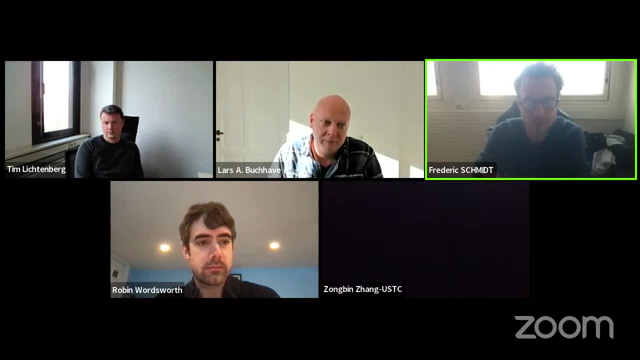 have to combine a different uh observation to have something for the atmosphere. i think. uh. well, i'm not a i'm not a real expert on moons, but i know david kipping very well. i was sitting next to him uh for some years in the in the office next to him at the cfa and i mean i think 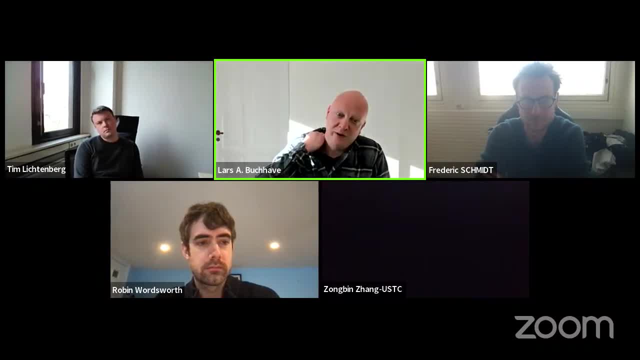 my understanding is that large exo moons are not- i've sort of been ruled out- uh- that like like the size of the earth or something like that. so you really have to. exo moons are extremely, extremely difficult, um, and so i think you know, just detecting an exomoon or characterizing it, But I'm not an expert, but I think it will be. 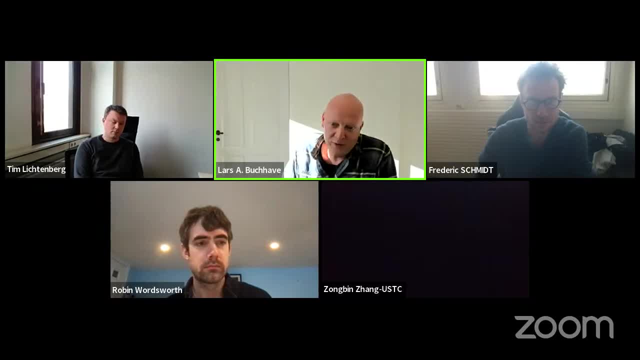 very difficult. They are very small. If you look at the moons in our solar system, they're just so much smaller and more difficult, So it may be very difficult. Okay, so the Earth's moon size, for instance, would be completely out of the signal to noise. 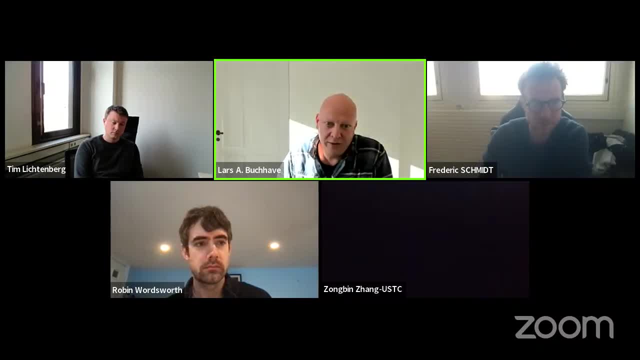 to detect, I think so. I mean, what David did, I remember, was take, for example, many of the Kepler planets systems and sort of stretch the transits to allow them to stack multiple systems on top of each other, And then if there were moons you might see sort of a little dip before. 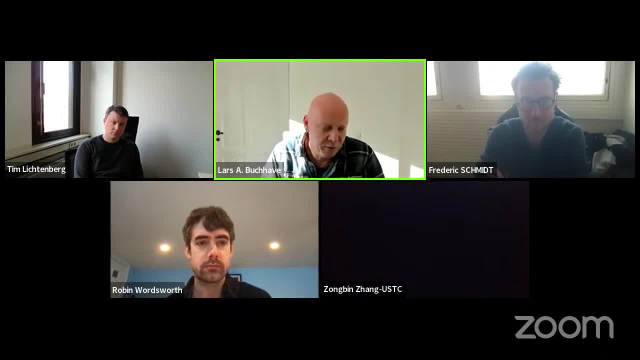 the ingress And he has some upper limits there And it rules out very large moons at least Sort of the same size of binary planets or something like that, And so it's really, really difficult to detect moons. Okay, thank you. 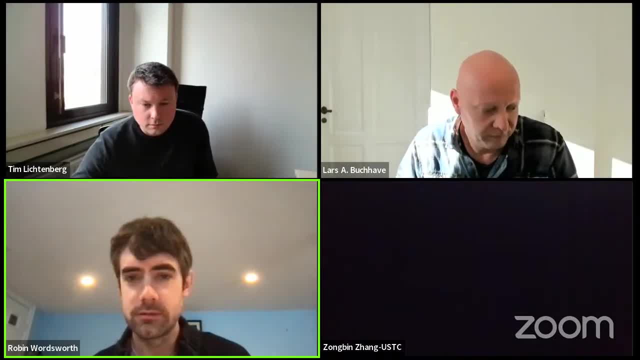 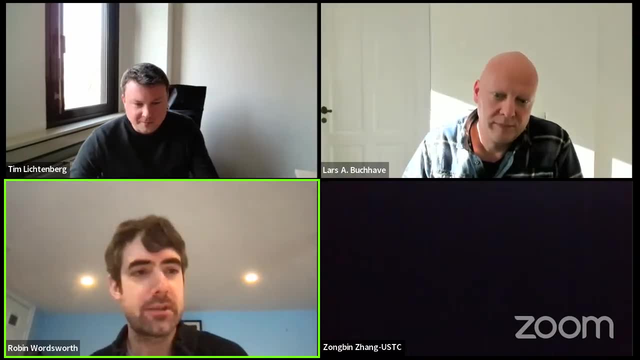 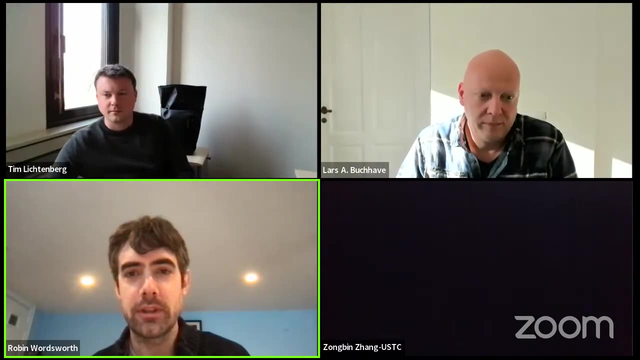 Additional questions for Lars. So I guess I have one about the TRAPPIST-1c observations that you're doing, Obviously initially just looking for any kind of detection or non-detection of an atmosphere. But I saw you were simulating 10 bar O2 atmospheres and also CO2 atmospheres. 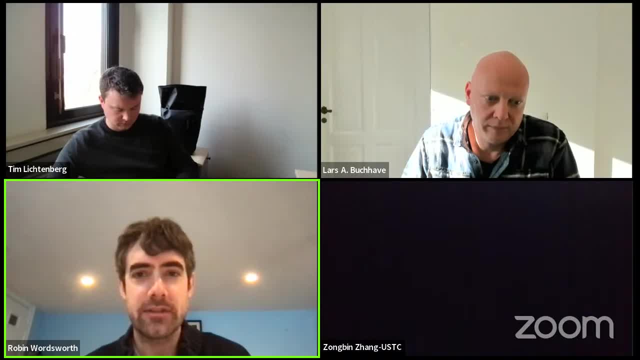 Am I right in understanding that you're not going to be able to detect O2 directly? It's just going to be background gas in this sense? So you're looking for signals of CO2 or possibly H2O? Yeah, O2 is out of the question. This is: yeah, it's just as a background gas, So it's a CO2 trace. 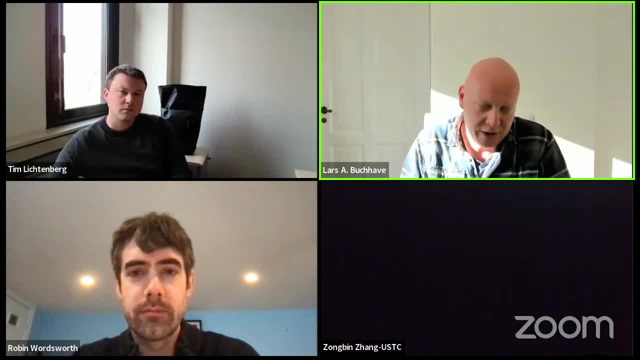 gas in an oxygen dominated atmosphere is what we were. I think it's from, is it Lindkowski? I think that did these simulations. I believe O2 collision induced absorption doesn't help you at all in that. in the James Webb spectral range. 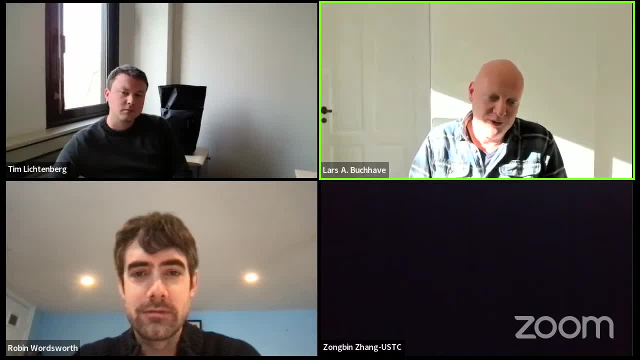 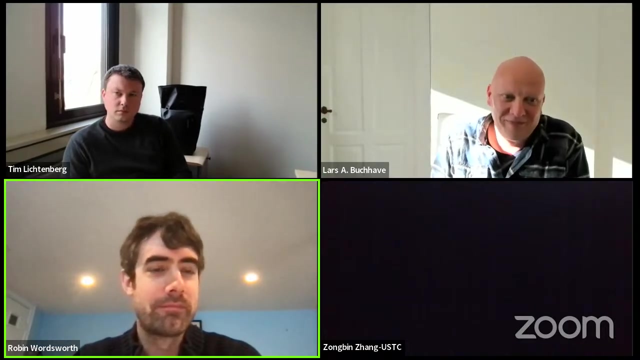 I don't. It's very difficult to do to take those through. And the main, the main features, is just in the very, very blue part of where you see the uncertainties explode in the background. So you can't see them there, you can't see them in the background And you can't see them in the 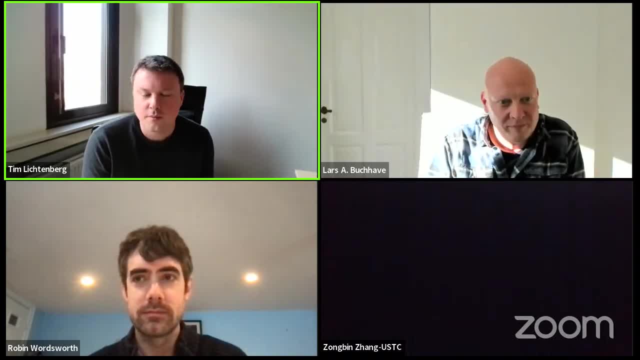 prism data, So that's going to be extremely difficult. I would be happy if you see any species at all. Right, Yeah, that's obviously the primary objective, Tim. Yeah, a follow up question on that. So with the data you've got already, can you sort of better? 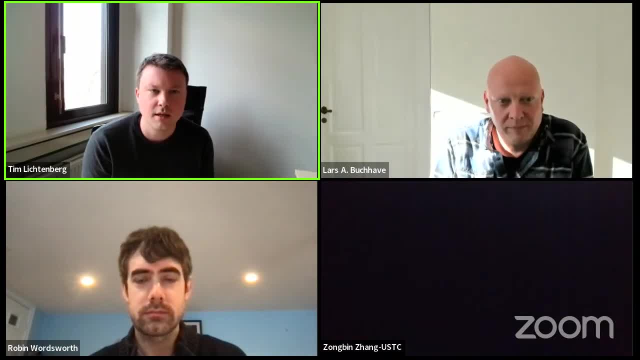 understand, with the following transits that are already scheduled, how that the data acquisition, the first measurements, were taken. Can you refine or can you already see how the follow-up measurements, how far they will get you? Yeah, so are you talking about signal-to-noise? 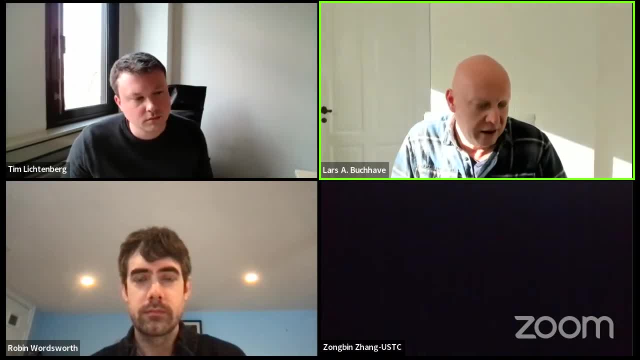 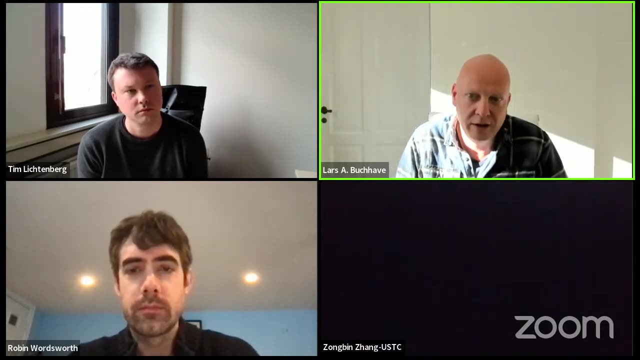 or are you talking about? yeah, So I mean, barring stellar activity and no atmosphere and things like that, and also systematics that you're unaware of, just a pure signal-to-noise is actually better than the simulations predicted, And so that's really encouraging. 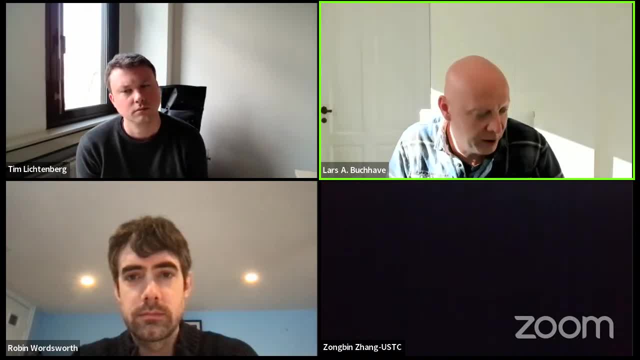 I think most of the instruments are actually performing better than expected on the internet, And so, with that in mind, I think we're actually going to get better signal-to-noise than we simulated. Of course, then there's all the things that you're not aware of. 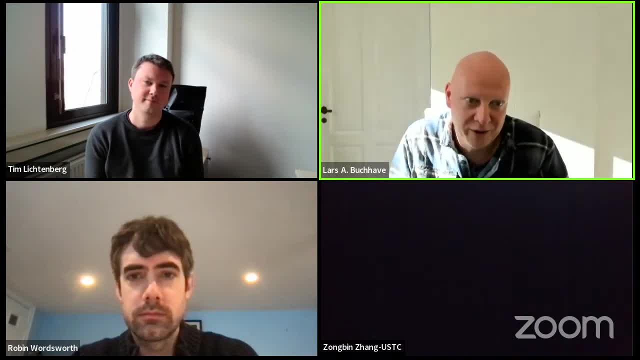 like systematics or stellar activity and unocculted spots or all these things that can make it much more difficult and trap this. This is probably a somewhat active star. The initial observations indicate some of the we see slopes in some of the other transits. 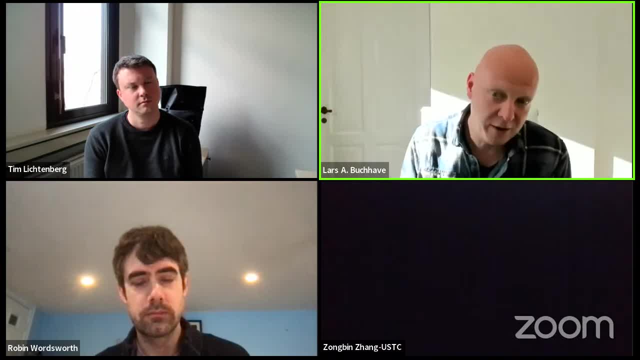 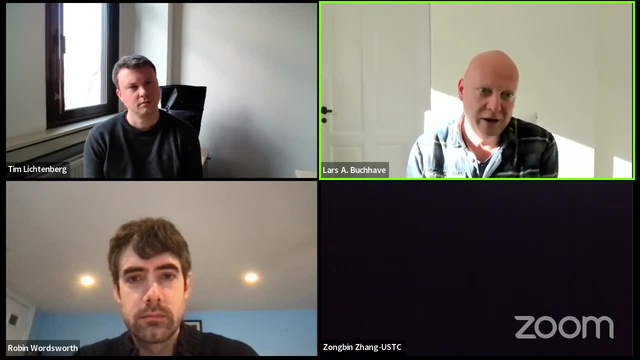 that have been observed, not of our data but in other, and some of the other transits are completely flat and with no stellar activity. So I think that's probably going to be the main issue And, of course, then the next question. 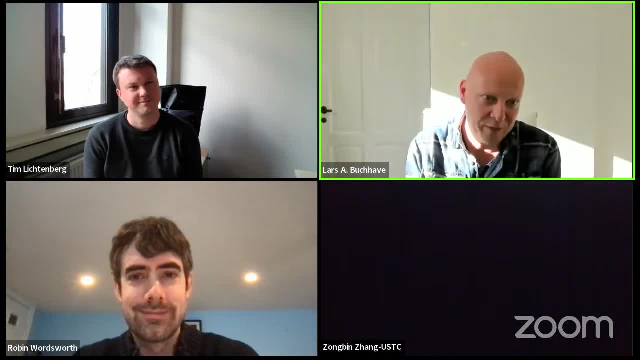 is whether these planets even have atmospheres at all. I know Lord Kreitberg has a data set on trying to also look at trappers, but see that it has been observed, So I think that's probably going to be the main issue, by doing secondary eclipse measurements. 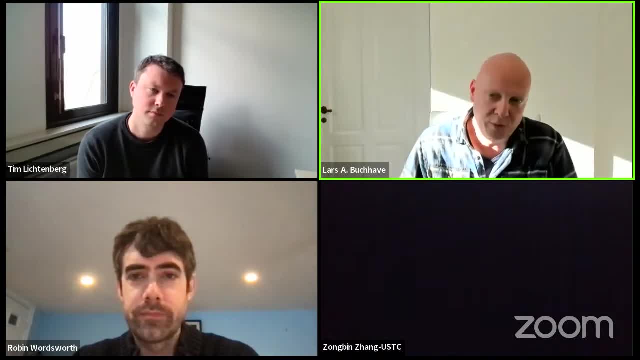 and looking at whether there's heat distribution of the atmosphere and thus trying to look at the binary question: is there an atmosphere or not? And those data have also been taken, So the word is still out, but we'll see whether these planets have atmospheres. 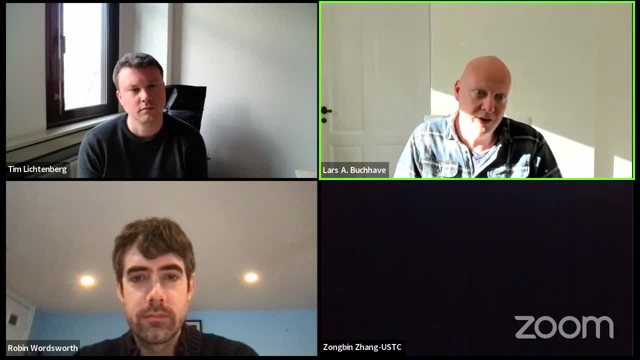 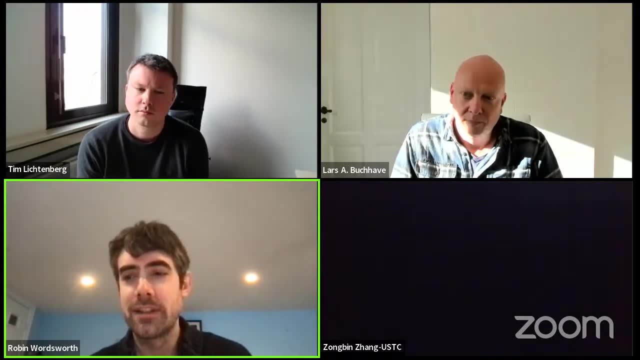 But I think the data looks very encouraging in terms of signal-to-noise really looks encouraging. Yeah, and to follow up on that a little bit, this is kind of a question about unknown unknowns. but if you were for the general audience, 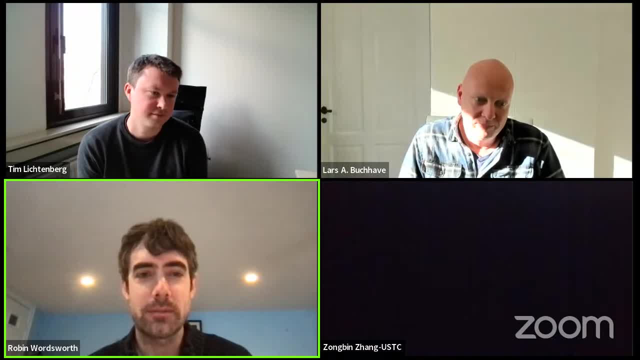 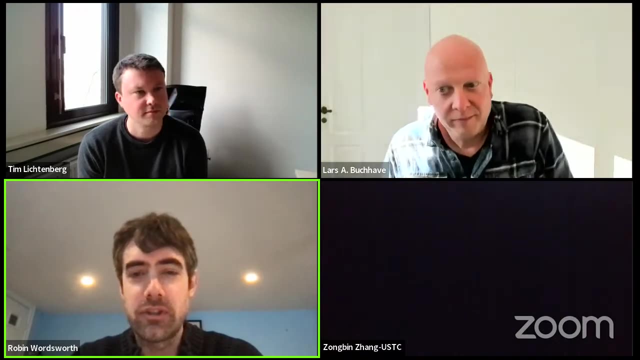 to say how you think the systematics evaluation is going to develop for James Webb and what we should expect going forward? do you feel optimistic generally that the kind of initial problems we're seeing now are going to lessen as understandings of the instruments improves? 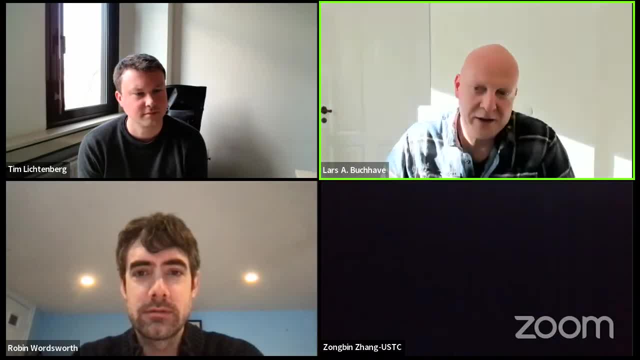 Yeah, I think the general community feeling is that it's actually very well behaved And there's very- I mean, compared to maybe Hubble, there's much fewer systematics And the community has also really come together to put together a number of different pipelines. 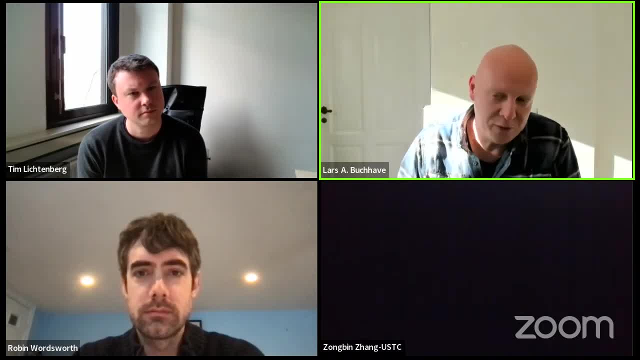 to look at this. The trouble with our observation in particular is that we have this extremely small server rate, which we chose due to cadence and signal-to-noise. We basically just try to optimize as much as possible and get as many photons as possible. 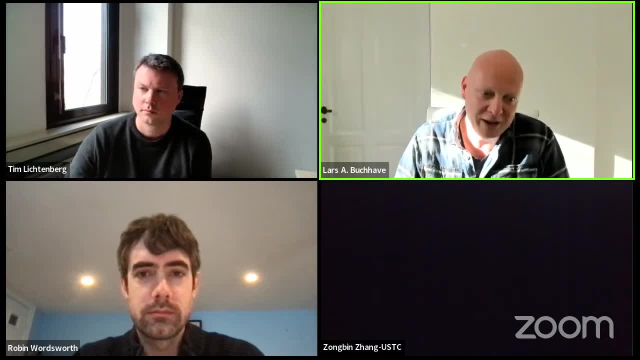 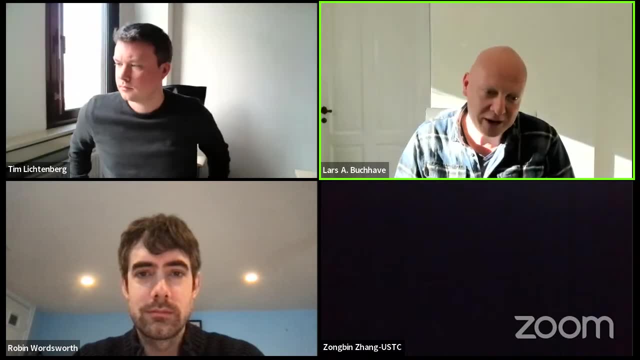 But then now, being wiser and looking back, we may not want to use this very narrow server rate, because there's a number of data reduction issues and systematics that are difficult to deal with when we have this very narrow- As you saw in one of my plots. 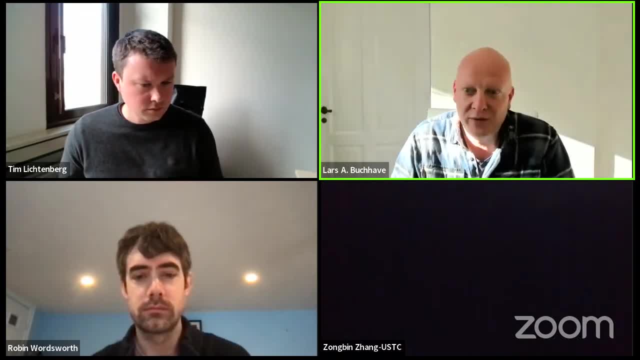 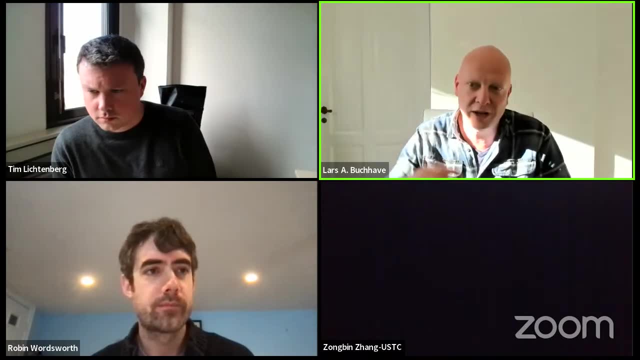 the flux actually spills out over the edge of the detector And that's so. we're kind of it's very little, but we're still not capturing all the photons that we're getting in, And so when we're trying to, for example, 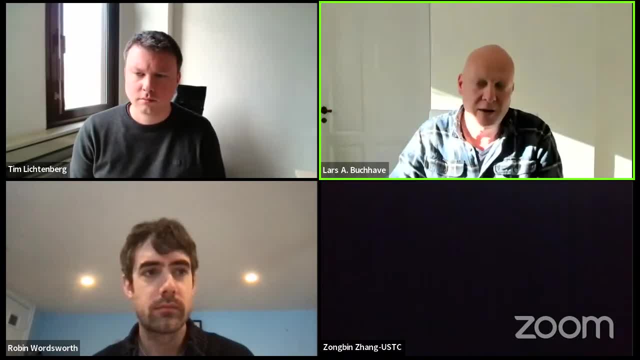 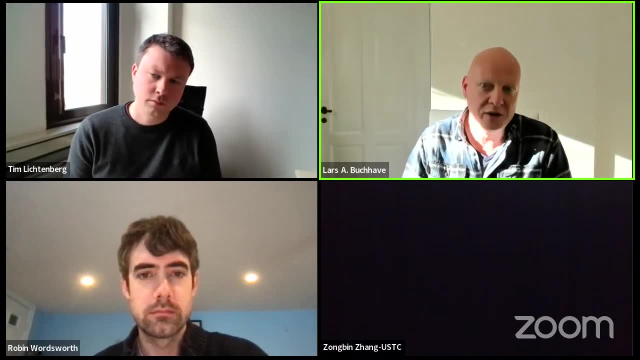 remove systematics like this one over F noise, which is basically read detector noise that changes from column to column. that makes it very difficult. So I think general consensus is that we're that we will have the systematics under control, but we need to understand which instruments. 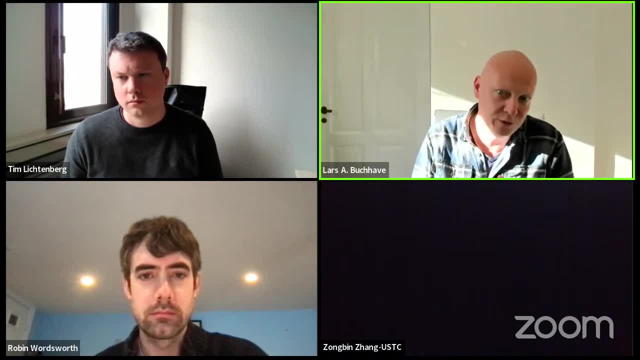 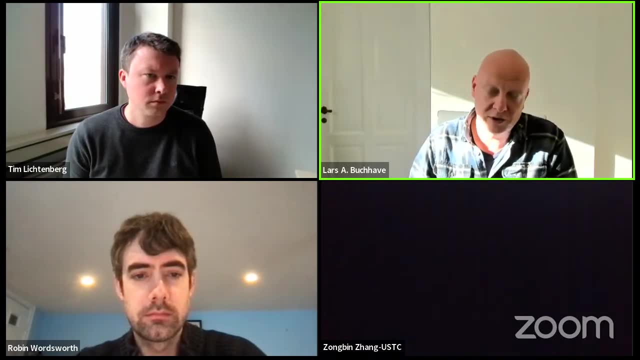 and what modes are the best for these observations? If we go to different subarrays for a planet like TRAPPIST or a star like TRAPPIST-1,, there are data points that will completely saturate in the spectrum, And so, for example, 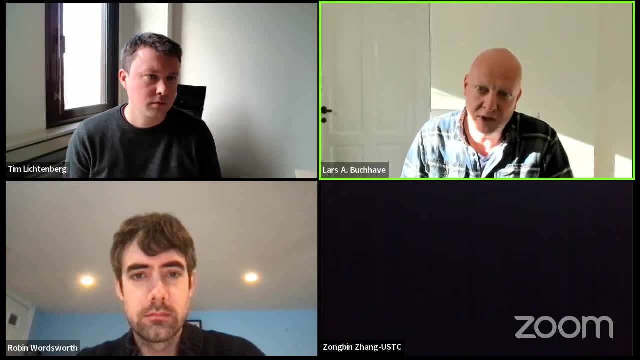 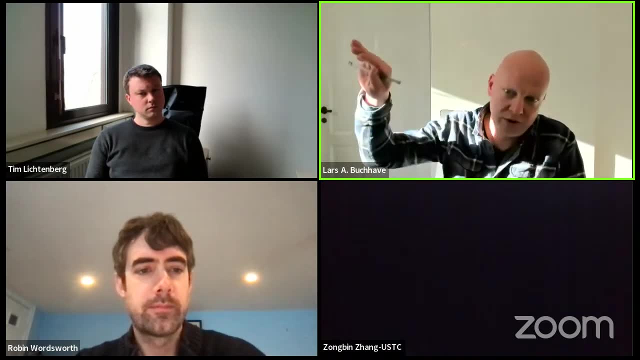 I know that there's observations of TRAPPIST-1G with the near spec prism instrument and they chose a different observation strategy where they're doing- we're doing- three: a ramp of three reach outs and then a new integration. 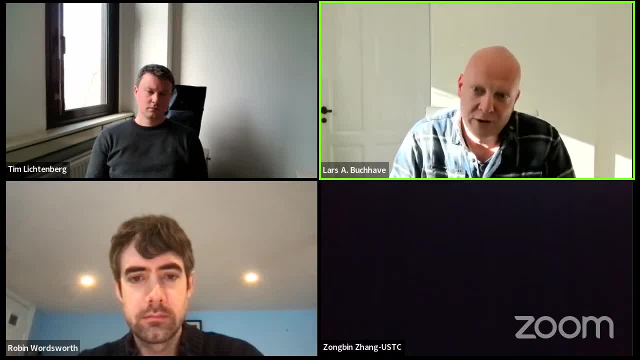 They have six And so in the peak of the flux they will saturate many of those ramps And also they have a slower readout because they have a larger detector. But I think perhaps that is a better way to do it actually. 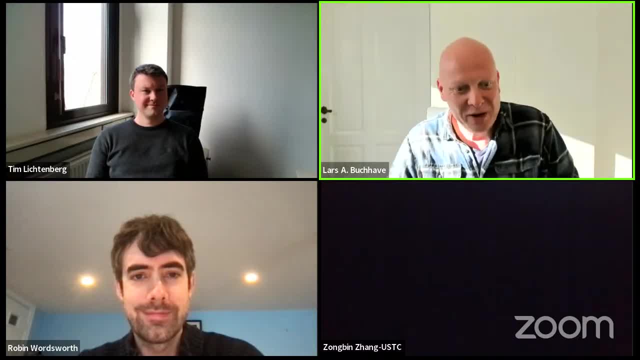 That wasn't our initial assessment, but now that we're looking back, there's so many unknowns when we're writing proposals and trying to configure them without knowing all the details. I hadn't even heard of one over F noise at that time. 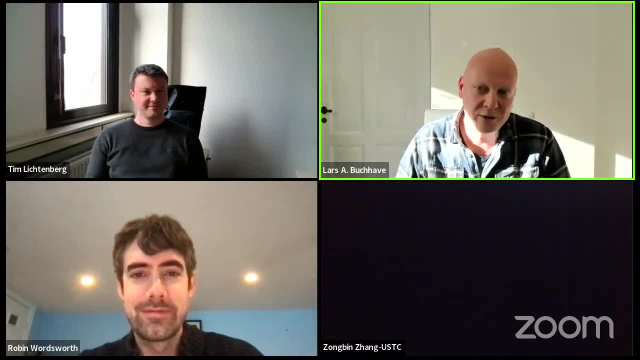 So I wasn't even aware of issues we really had to do, But I think the general sense is that was a very long-winded answer. sorry, but is that the systematics are, we'll be able to get this under control. 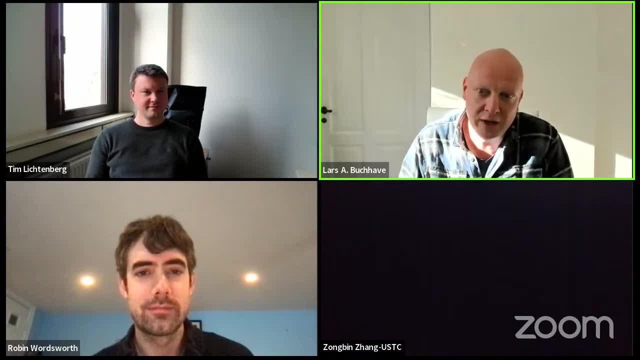 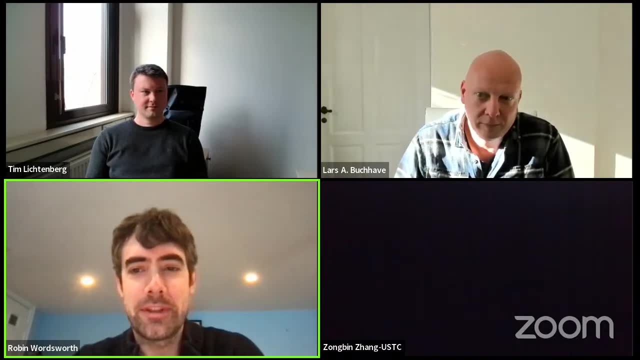 And I think we'll then optimize what what we're doing And that's what kind of modes we'll be observing, and that will give us the best data. Yeah, thanks for the response. It's interesting to hear how things are evolving so quickly. 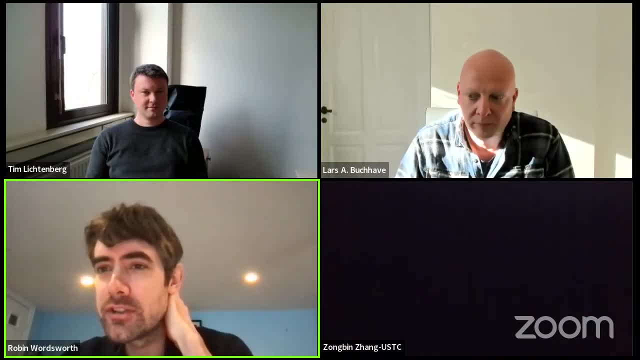 We've got a comment from Nick in the chat as well. I think a comment rather than a question. He says repeat observations are definitely key. James Webb is operating beautifully, but Trappist-1 is constantly messing with us. No, two observations are exactly the same. 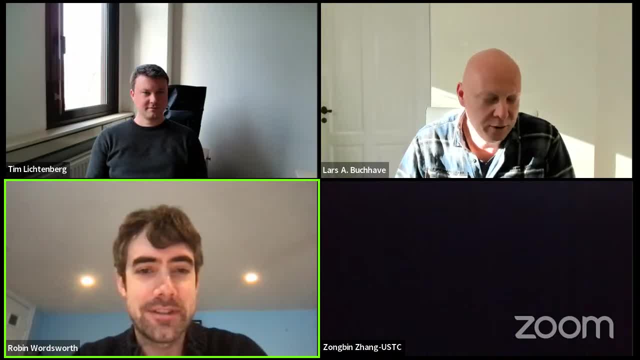 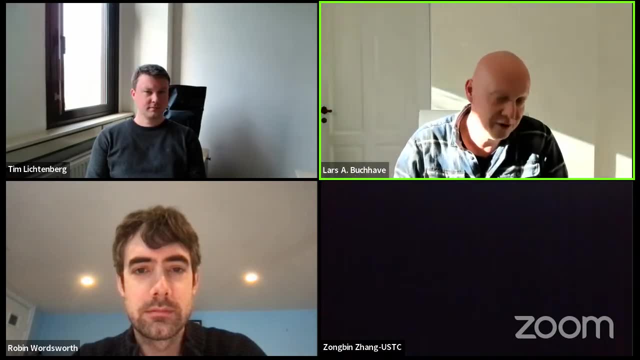 So stellar activity obviously always- Yeah, I know this, but there's community efforts to try to really there's a proposal, I believe, that's trying to stay on data- maybe, Nick, you're a part of that- to really stay on Trappist-1. 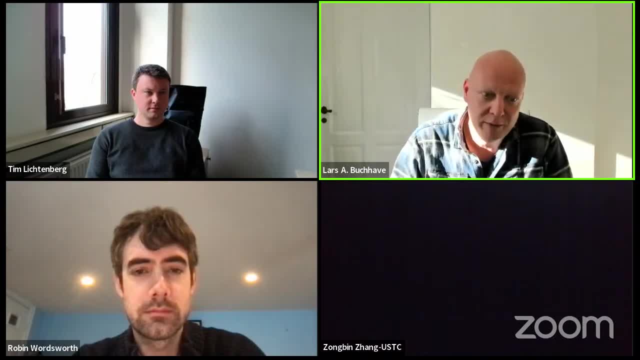 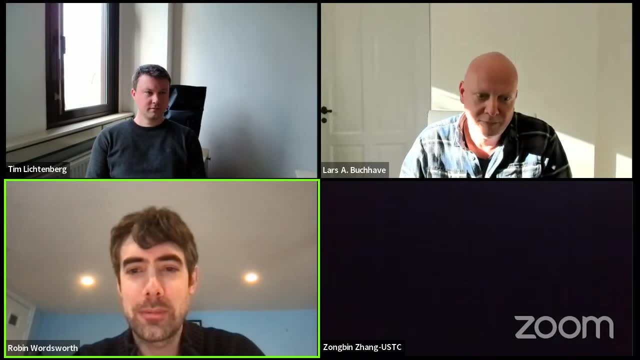 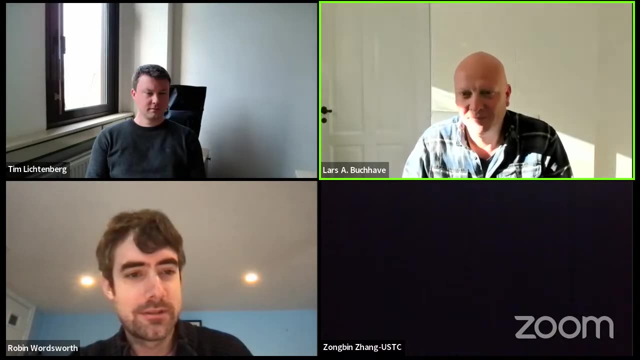 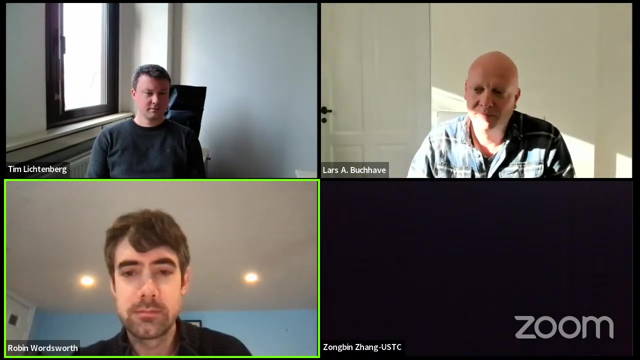 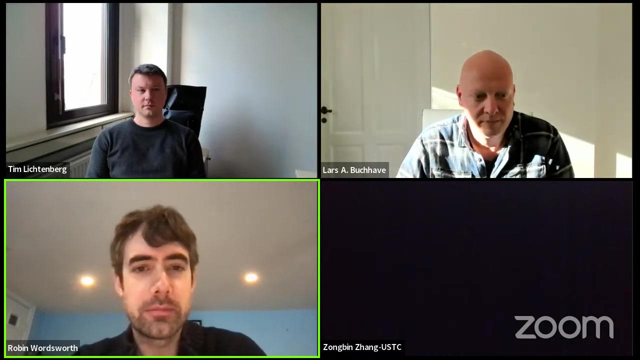 and try to really understand the stellar activity with James Webb. So that's definitely going to be important And dwarfs both opportunities and challenges. We have further questions for Lars, So I guess one more thing I could ask on the more on the sort of observation versus theory side. 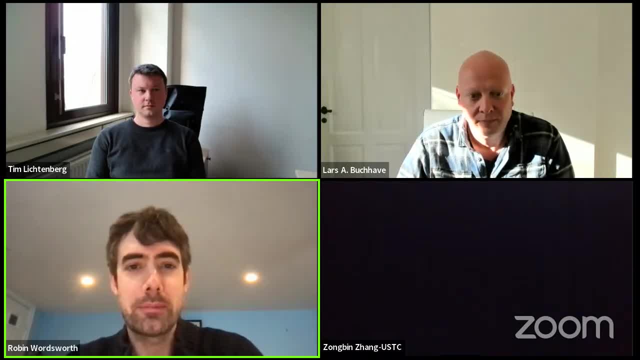 it kind of as observers. of course you have the luxury of just looking at something and seeing what you find and that drives the theoretical development. but I'm curious nonetheless for the Trappist system, if you, if there are sort of specific atmospheric loss. 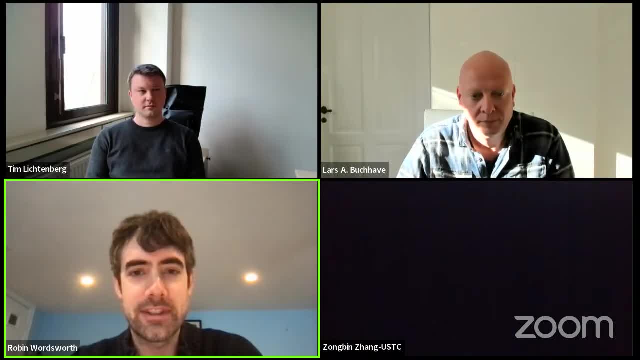 theories you're thinking about comparing with or processes that you think may be most important in that system for determining the line between airless bodies and those that retain some atmospheres. Yeah, I that's a good question, but it's really I think that's a tough question. 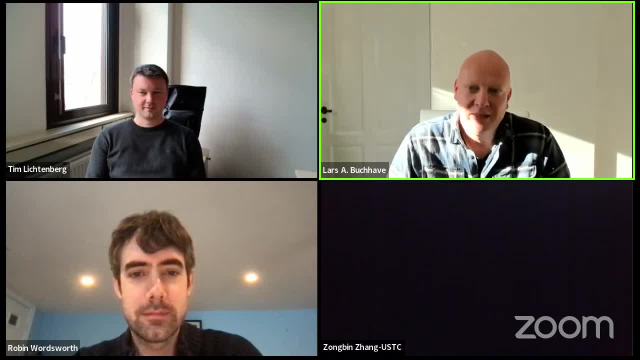 because I think we know so little at this point that you know taking the first atmospheres will be really important to figure out which directions to go. So another thing we haven't discussed is clouds in the atmospheres of these planets. that's of course a major problem if all these small planets 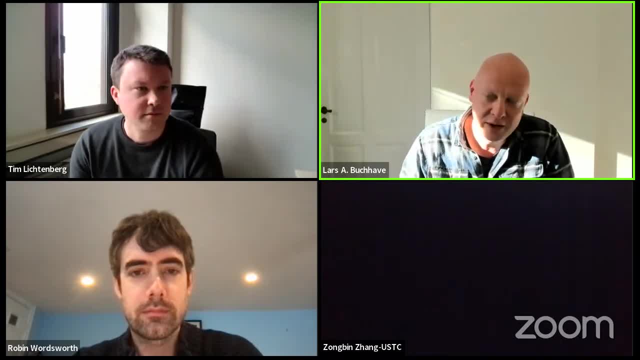 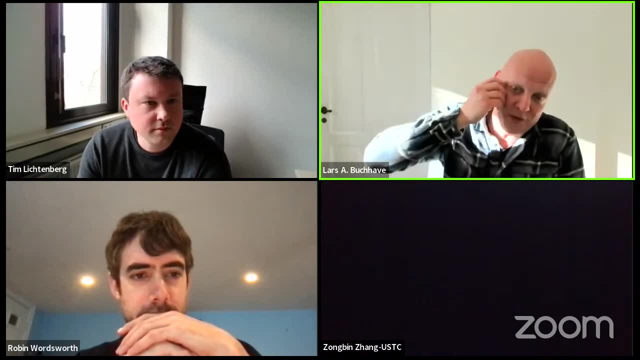 or exhibit like high clouds or hazes in their atmospheres, And so that our program was tailored to detect an atmosphere if it's rather a clear atmosphere. Now, if it's a cloudy atmosphere, it would be excruciatingly hard to do. 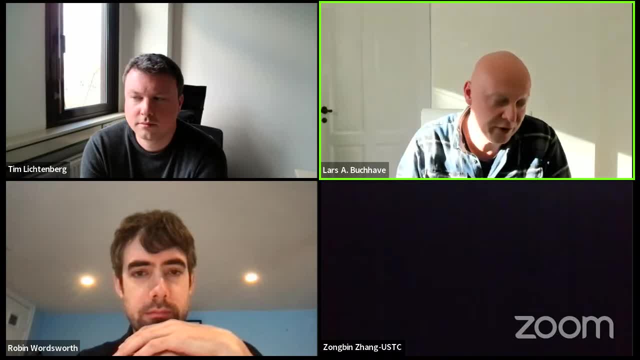 and require many, many more transits than the four that we've asked for for TRAPPIST-1c, And so our philosophy was: let's try to see if we can detect clear atmospheres around these planets. If not, then either there is no atmosphere. 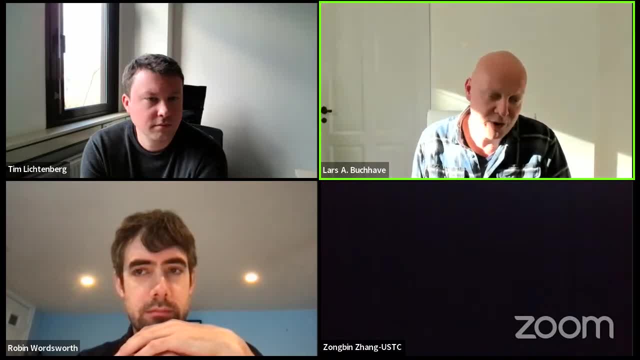 or it's a very cloudy atmosphere. In either case, there will probably be more interesting targets to spend the precious JWST time on, because if they're very cloudy, it just requires so many more transits to even begin to detect any atmospheric features. 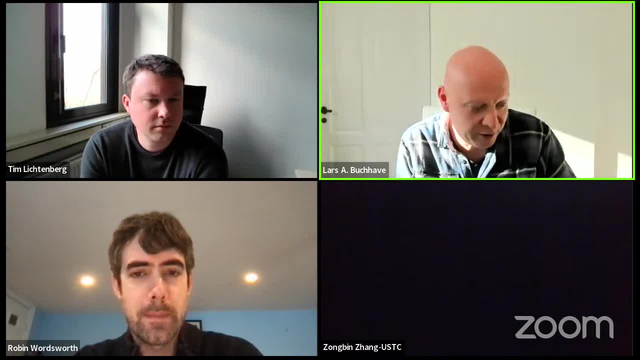 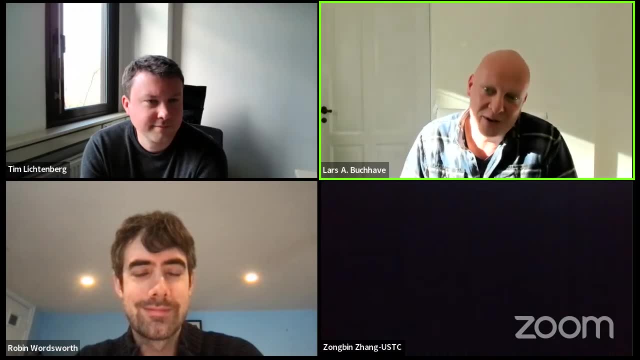 So I think to me the time now is to find clear atmospheres on terrestrial planets, if they exist, and try to characterize those with the precious time we have with JWST and sort of find clears, find those fantastic planets that we can actually do some characterization of. 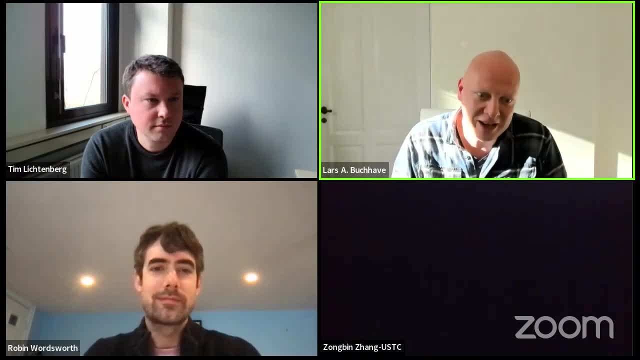 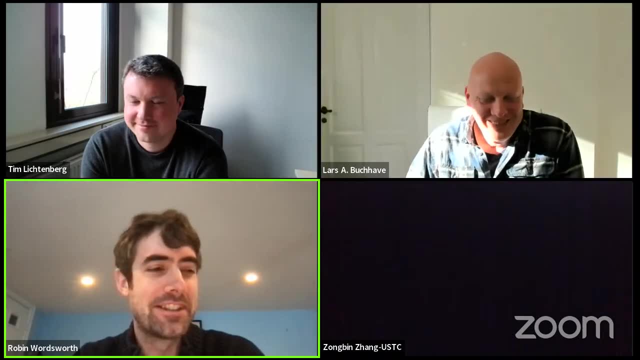 I don't know, That's not a very good answer to your question, But right now I would ask you the question. Robin, actually That question you posed me really. In fact, I was just about to respond by saying it would be wonderful if theory could give. 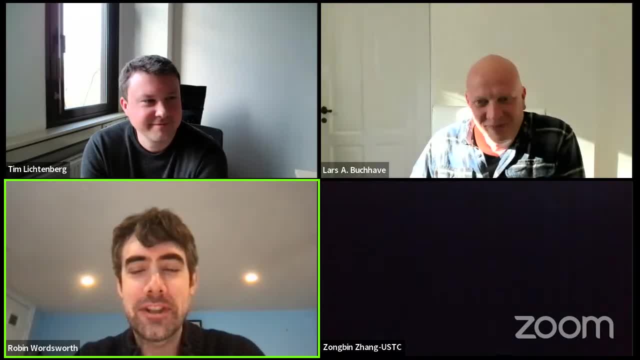 some guidance about where we expect clouds to appear or not, And there's certainly work being done to try to accomplish that. But clouds are, as everybody knows, an extreme challenge And I think even in some cases we're ruling out H2, HE atmospheres. 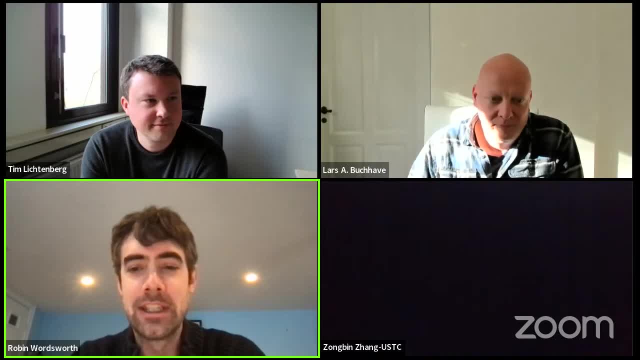 If the clouds are high enough, you're still going to have problems even then. So I suppose the solution is continued into comparison of theory and laboratory experiments. I think laboratory experiments in particular are really important because we just don't have some of the data in the range that we need, particularly for haze formation, right. 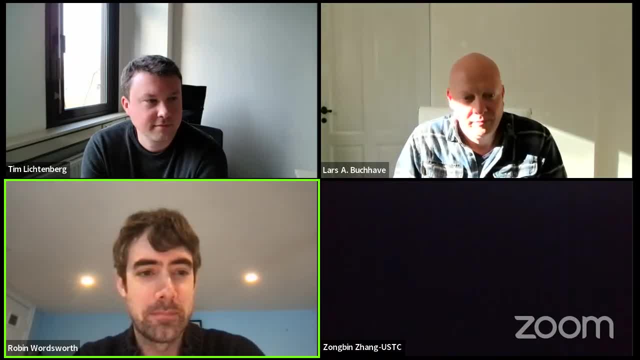 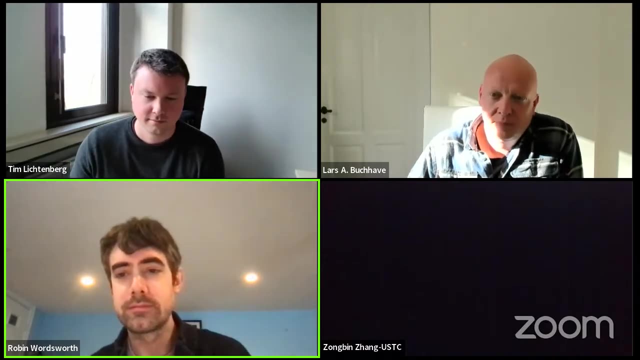 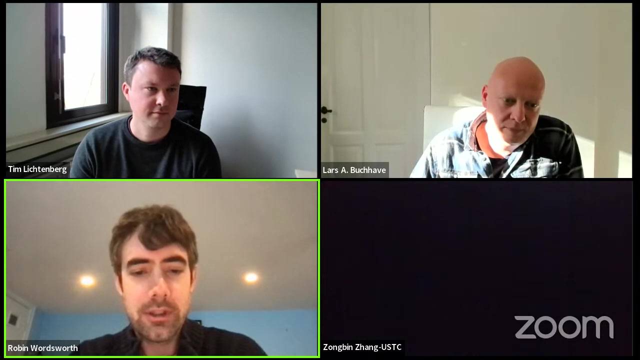 now. But, yeah, ongoing challenge for sure. If anyone has anything to add to that, Okay. Well, if there are no more questions or discussion points, I suggest we wrap up there And those of us on the East Coast can go and get some breakfast. 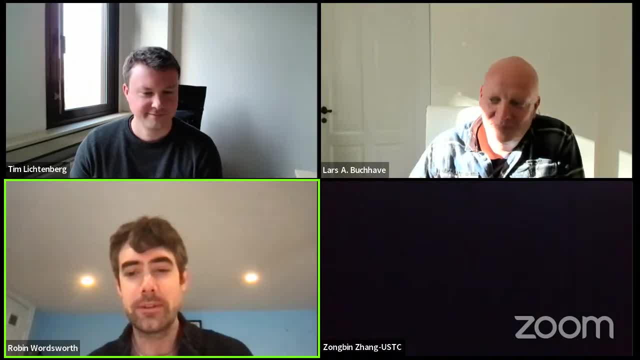 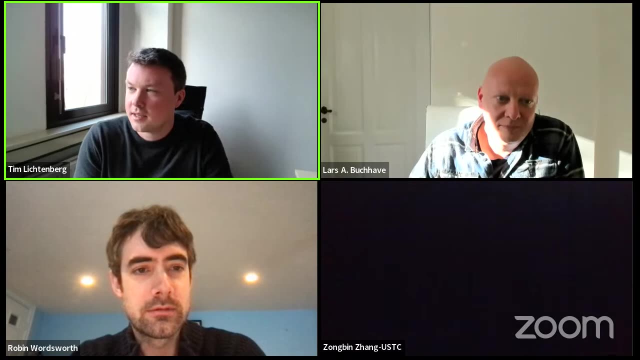 I want everyone to thank Lars again one more time for an excellent presentation, And Tim, I don't know. do we have any Rocky Worlds discussion-related announcements before we close? Yeah, I mean, the next seminar is on 6th of April, Thursday. 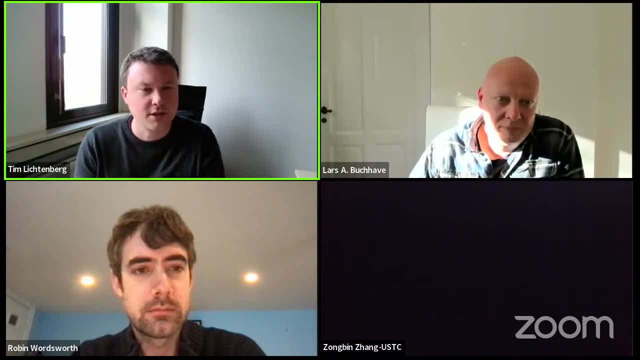 But the speakers Currently still in discussion, So we will announce this just using the website and mailing list. Excellent, All right. Thanks for joining everyone, And thanks again, Lars, Okay.